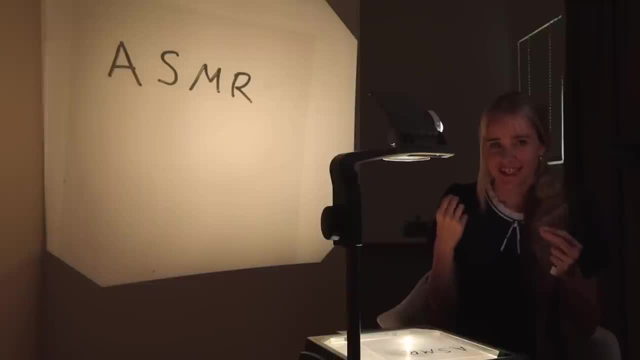 when you're listening with headphones in. it can give you this slightly tingly feeling in the back of your brain. I'm not sure if you've heard of ASMR, but it's a very popular thing. It's a very popular thing and so that's why people like it too. Often these ASMR videos are really softly whispered. 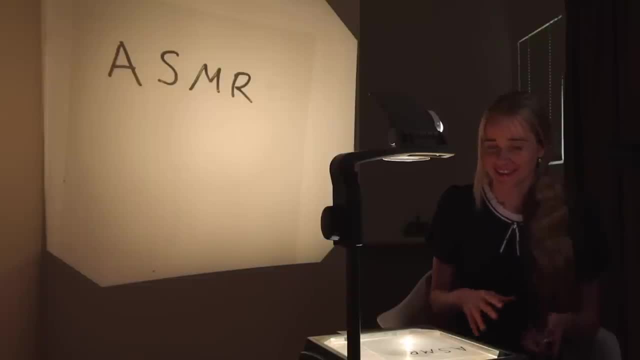 but I'm doing mine more soft spoken. One of the reasons for that is this projector makes quite a lot of noise. There's a fan in the bottom to keep everything cool and I'm worried that if I whispered too softly that perhaps you wouldn't be able to hear me very. 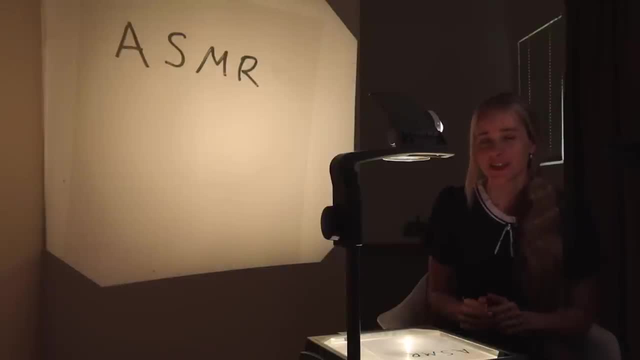 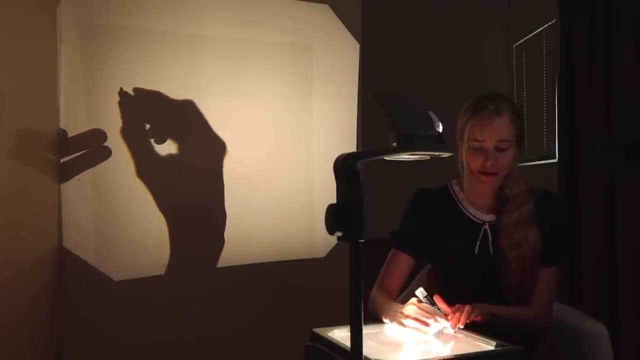 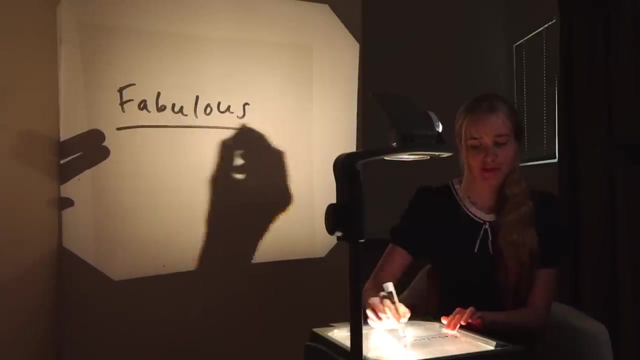 well over the sound of the overhead projector. I would like to quickly thank Fabulous for sponsoring this video. Fabulous is a pretty fitting sponsor for this video because they also place a lot of importance on relaxation, mindfulness and self-improvement. Fabulous is. 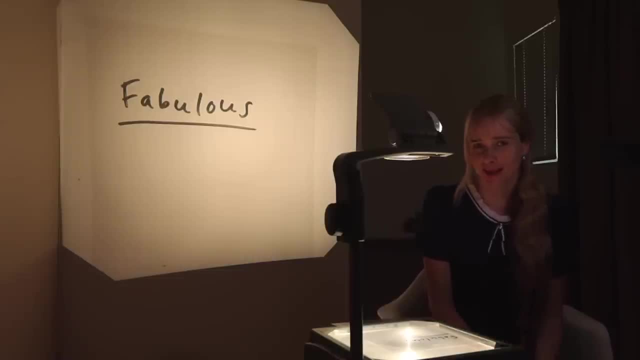 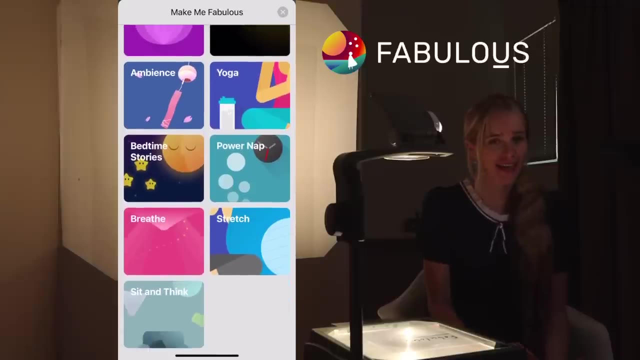 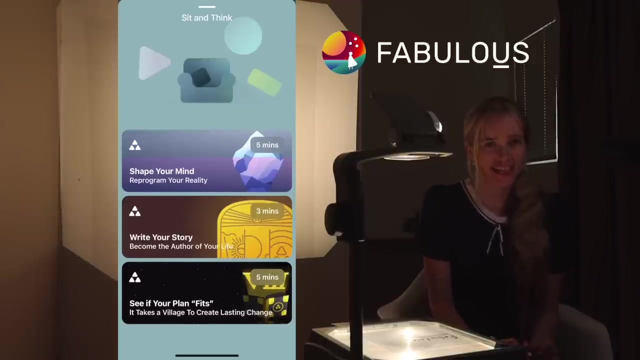 the number one self-care app to help you build better habits and achieve your goals. I think all of us have experience with setting new year's resolutions that get abandoned pretty quickly. but the best way to actually achieve your resolutions is to break them down into tiny habits, and the Fabulous app can help you stick to them. It was developed. 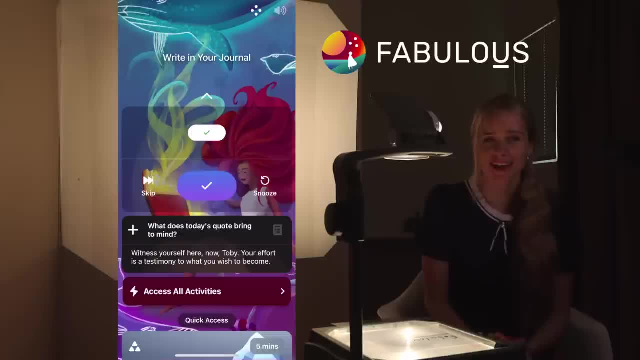 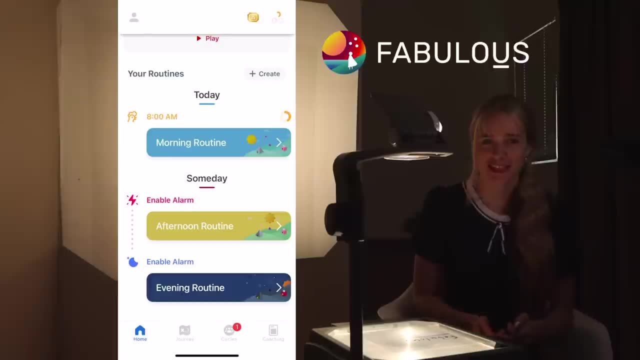 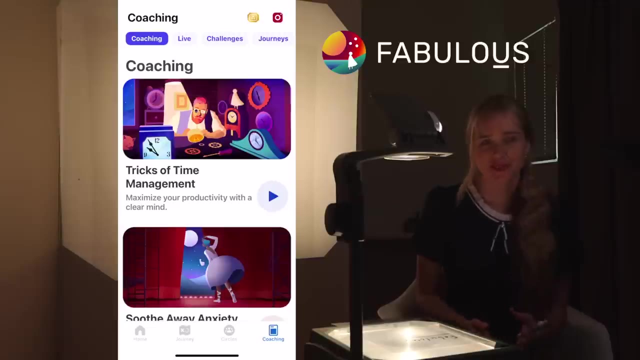 by behavioral scientists at uc university and contains guided journeys to help you achieve your goals. I've been using it to try and set up a morning routine that gives me a bit of momentum for the rest of the day, which I find can make all the difference. There's no shortcut to 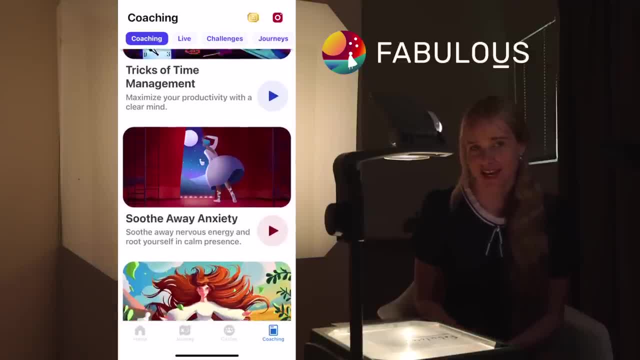 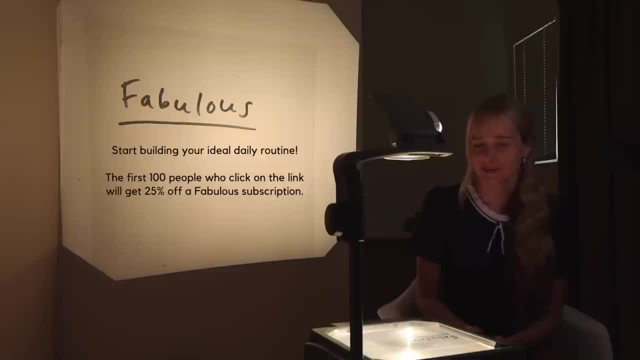 changing habits. but Fabulous offers a sustainable, long-term approach to change your life by building on small successes To start building your ideal daily routine. you can click on my link in the description and the first 100 people to do so will get 25%. 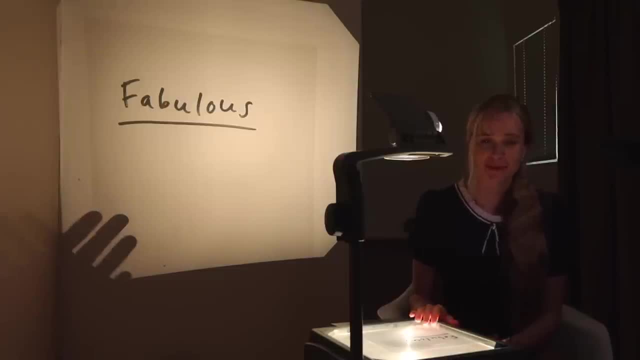 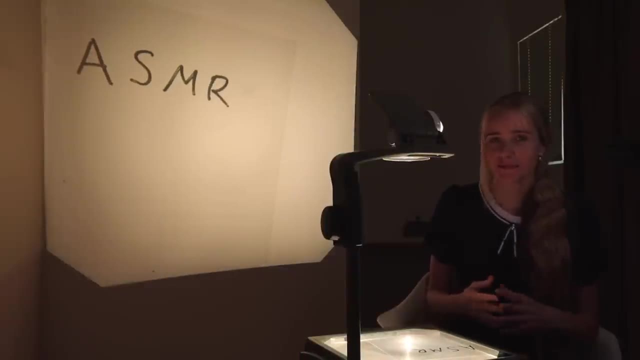 of a Fabulous subscription. So thank you to Fabulous and let's get on with the math. I have a plan for today to show you some math questions using the overhead projector, and for those of you who don't know what an overhead projector is, it's a sort of relaxing sort of. 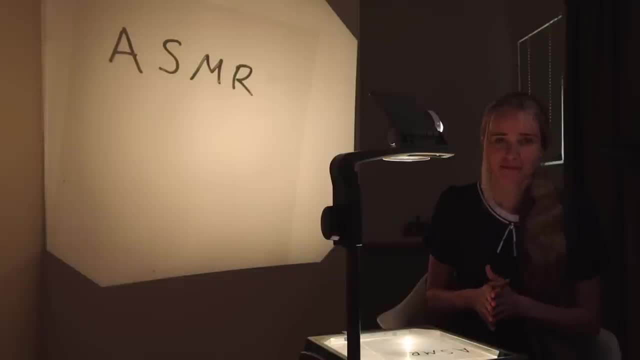 math lesson or overview. For some of you, math might induce a lot of anxiety, but hopefully this can be a way to boost your confidence or interest just a little bit in, you know, quite a relaxing setting. I've got exam questions from Brazil, Turkey, Australia, India, the UK and the USA and 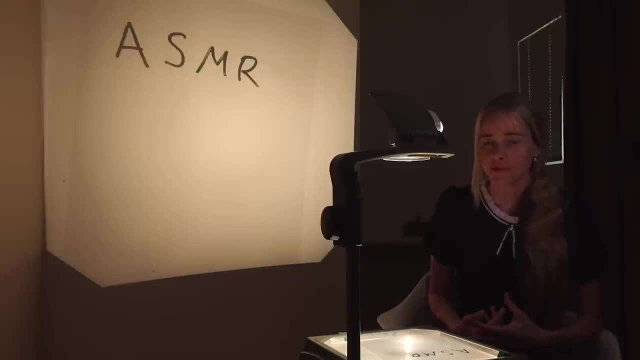 this video is going to be the opposite of the speed run. I'm going to be going through the questions slowly and in a way that I can talk about some of the fundamental ideas involved in the questions, so that, even if these things are quite unfamiliar to you or it's been a while since, 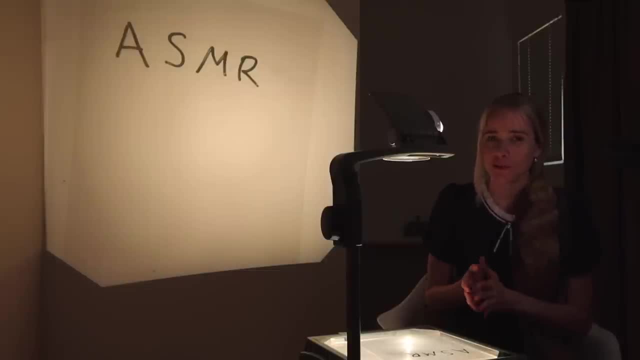 you did questions like these that you'll be able to follow along what's happening and what some of those fundamental ideas are behind it. A reason that I've picked exam questions to go through is for me personally. I've always learned quite a lot from watching problems get solved. 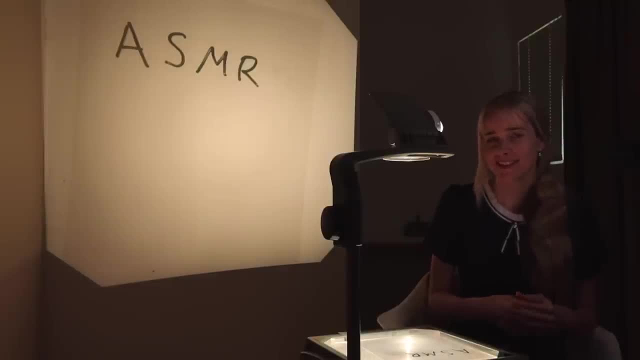 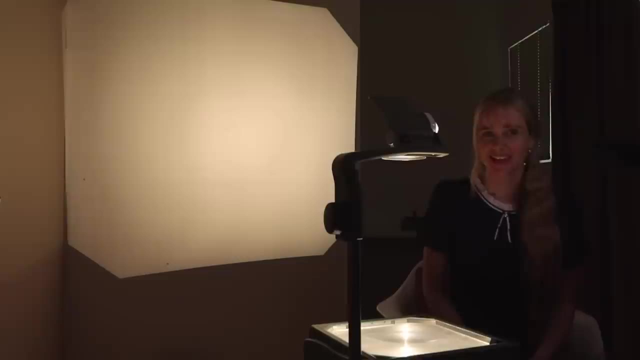 Compared to. you know, just reading about the fundamental ideas, seeing them actually in action and used in a problem, helps me understand their context a lot better. Our first stop is Turkey. This is a question from the 2021 AYT exam and, like many of the questions that I've chosen for, 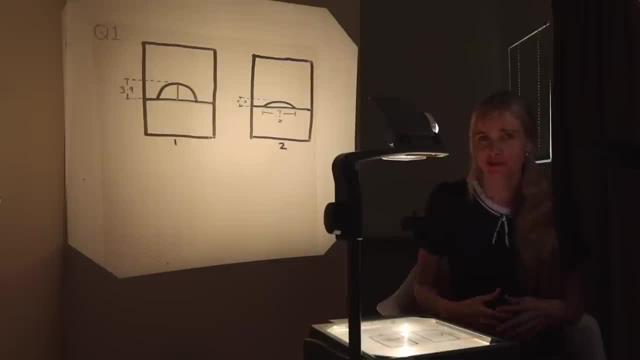 this video. it's for kind of an end of high school level or people wanting to gain entrance into university. Now this question was translated and the wording was quite long, but essentially it said that we've got two photographs of the sunset. Now, in photograph one, the sun appears as a semicircle. This is the ocean down here, the sun. 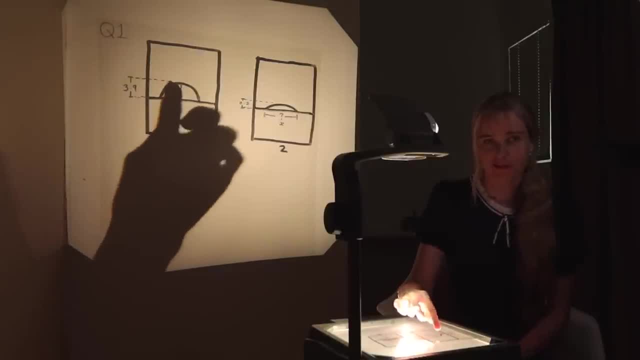 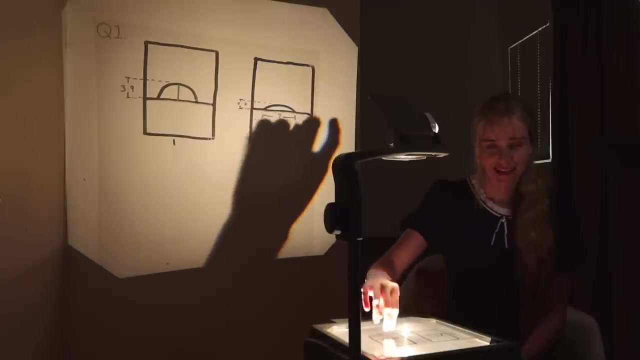 and then the clouds. Now the distance from the top of the sun to the waterline is 3.9 centimeters, as measured on the photograph. Then, after some undefined time later, we have picture number two, And the sun has sunk a little bit down over the horizon. and now the distance from the top of the 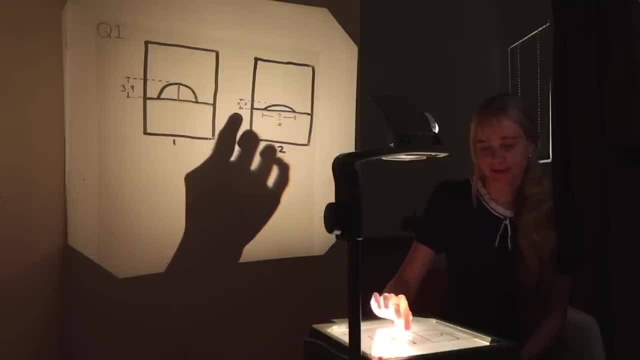 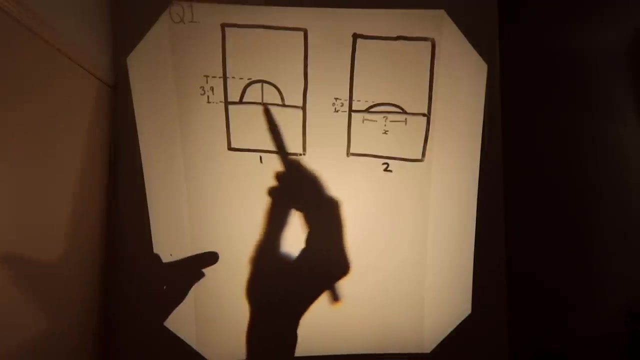 sun to the water is only 0.3 centimeters, as measured on here. Now what we want to find is this question: mark this mystery distance in here, which is how wide the sun appears in our second photo. A key word from the question is that this first image of the sun is a semicircle and a semicircle. 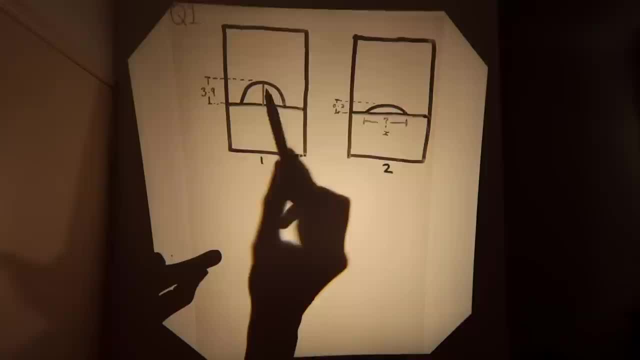 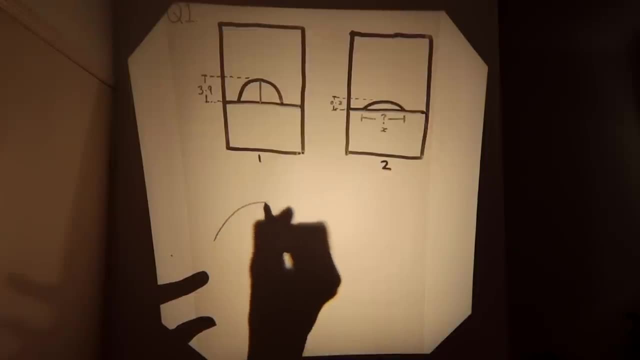 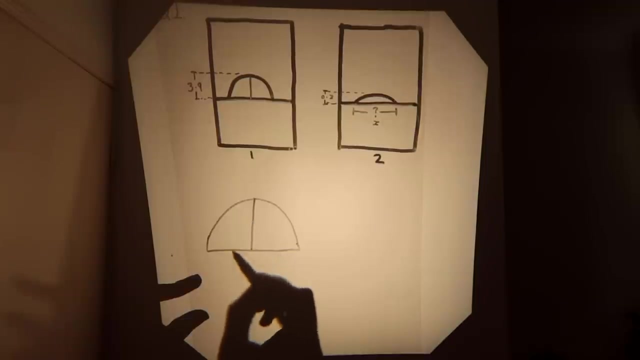 is exactly half of a circle, so that vertical distance that we're given is indeed the radius. So let's draw our own semicircle. From here we can mark what we know. If the sun initially looks like this, then after some time we just see the top of it. The distance in here was that given by 0.3. 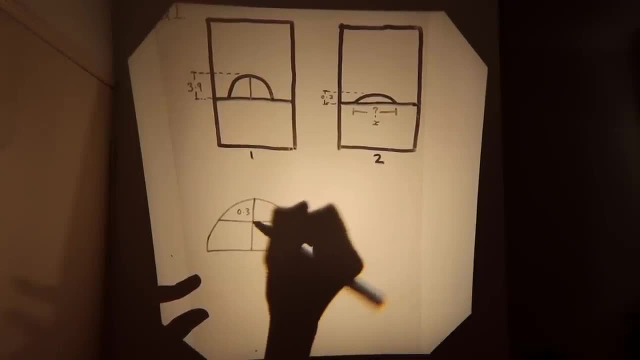 and this total distance we knew was 3.9, which means that if we take 0.3 off that, the rest is 3.6.. Our mystery distance is this line all the way across here, but since we've cut it in half, if 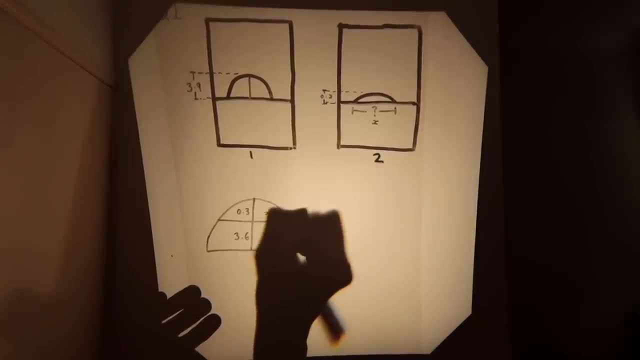 the whole thing were to be called x, this here would just be x over 2, and we can actually draw a right angle triangle right in here, Since it's a semicircle, and this distance was the radius. this line here is also the radius of the circle, so is also 3.9.. And with that we have a right. 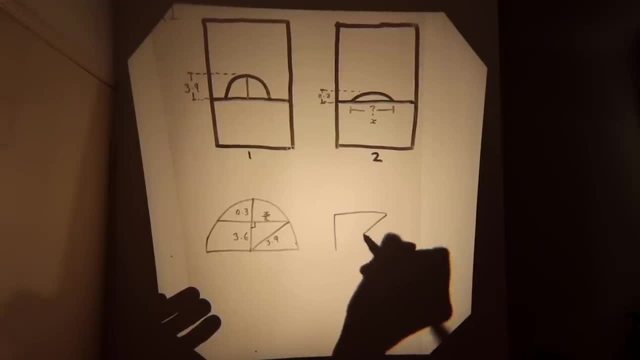 angle triangle where we know the value of two of the sides and we're trying to find the third side. For that we're able to use the pythagoras theorem. If this is our right angle triangle and one of the shorter sides is a, the other shorter side is b and the hypotenuse is c, then the pythagoras theorem says that: 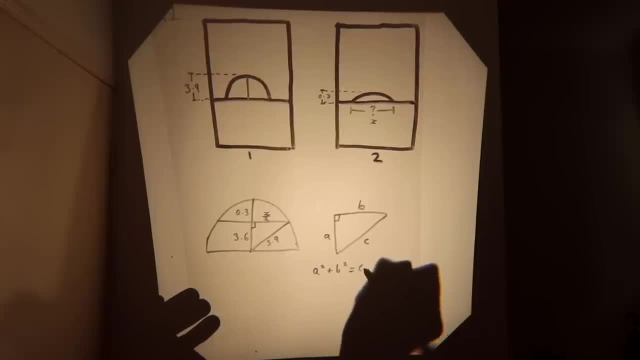 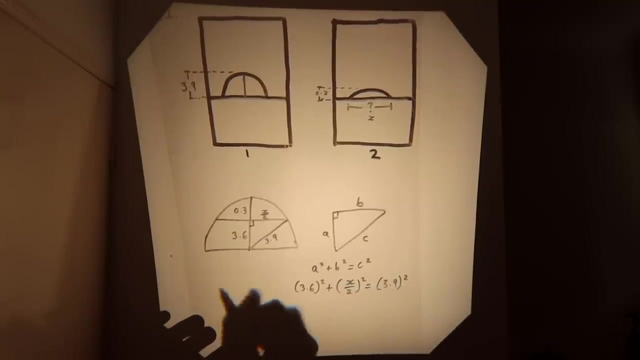 squared plus b squared is equal to c squared. For us a is 3.6, our b is x over 2 and our c is 3.9.. These decimal numbers are a little bit messy but it's not impossible to calculate these squares. 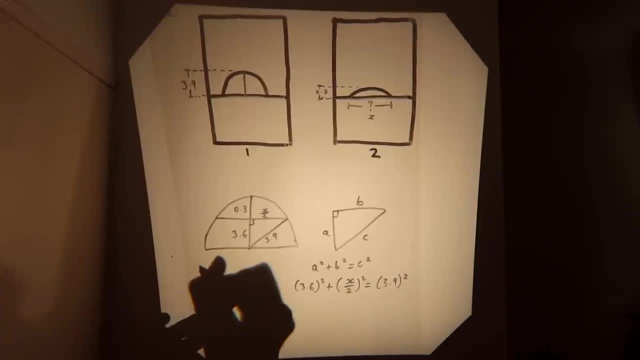 Remember you don't have a calculator for this question- We could go over to the margins and write 3.6 times 3.6. we could do: 6 times 6 is 36. carry the 3, 3 times 6 is 18,, 19,, 20,, 21.. 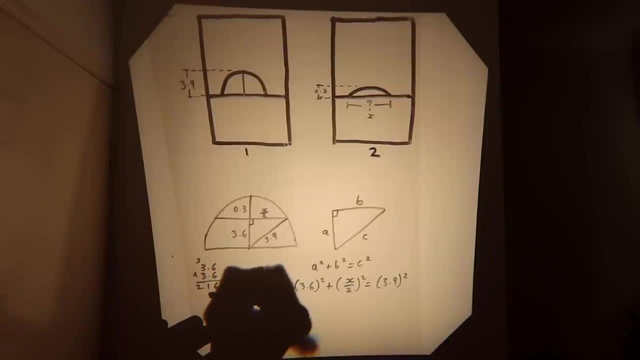 Add a zero here. go on to the next line. three sixes are 18.. Carry the one. three, threes are nine plus the one is ten. Add these up, we'll get six, nine, two, one. two digits Pass the decimal place in here, so our decimal point will go between the two and the nine and 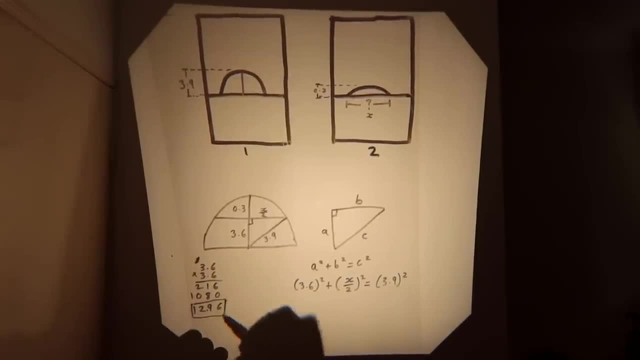 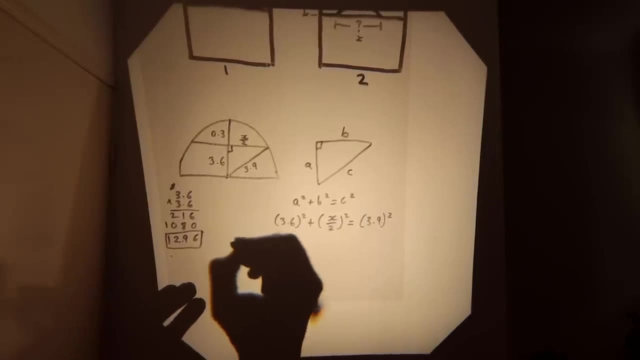 the answer to that would be 12.96.. Again, in our little margin, we could do the same to find 3.9 squared, We'd go 3.9 times 3.9, 9 times 9 is 81,, 3 times 9 is 27 plus 8 will give us 35.. 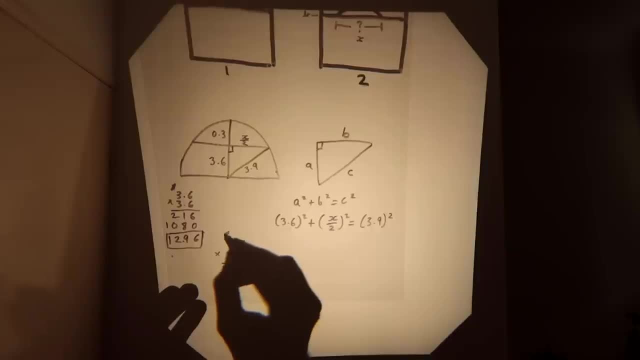 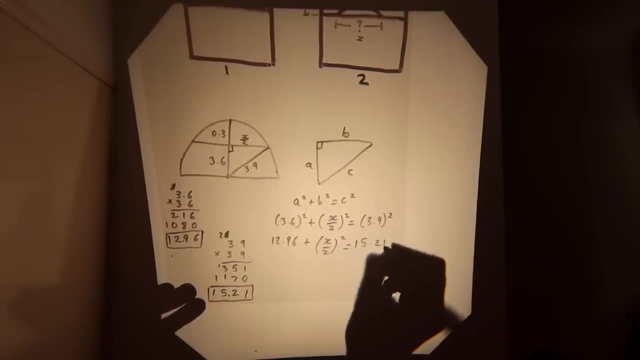 Do our next line: 3 times 9 is 27,. 3 times 3 is 9,, 10,, 11.. This one will add to give us 15.21.. So we've got 12.96 plus x over 2, squared is equal to 15.21.. x over 2. 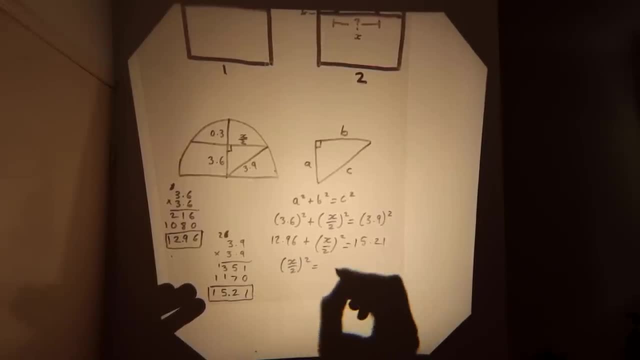 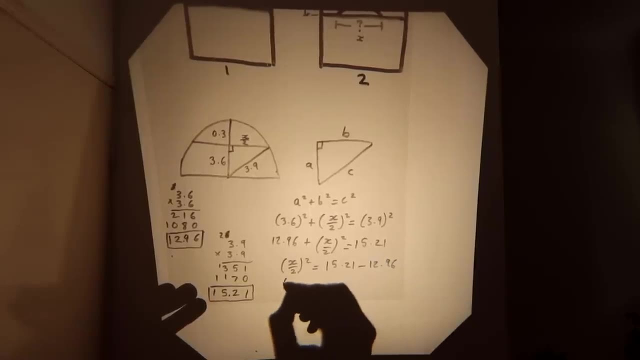 squared is equal to subtract the 12.9 from both sides. To mentally find the difference between these two numbers, I'd say: well, this is only 0.04 away from 13, and then 13 is 1, 2.21 away from this. so in total, the difference would be: 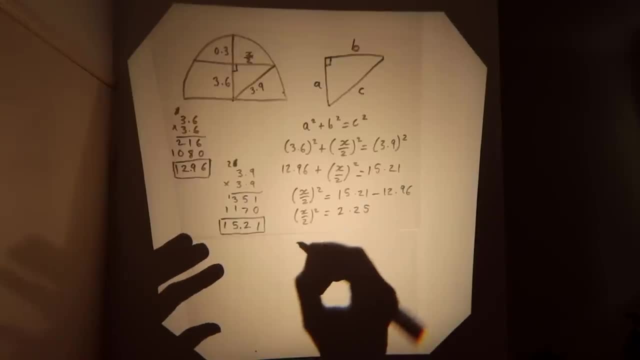 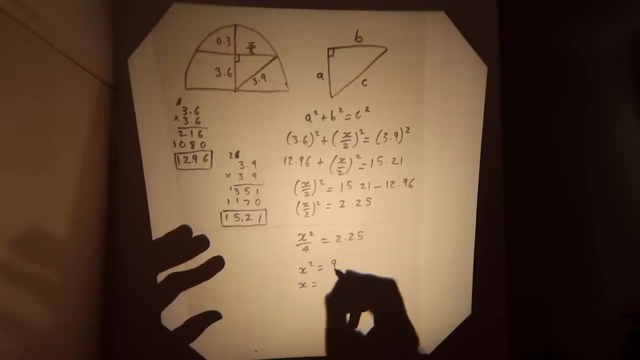 2.25.. x over 2 squared is the same as x squared over 4 times both sides by 4.. To get rid of this we have: x squared is equal to 9 and thankfully 9 is a pretty easy number to take the square root of, So I'm going to go with. x is equal to 3 centimeters. 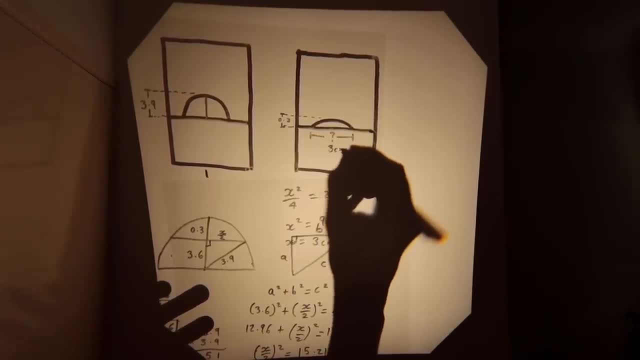 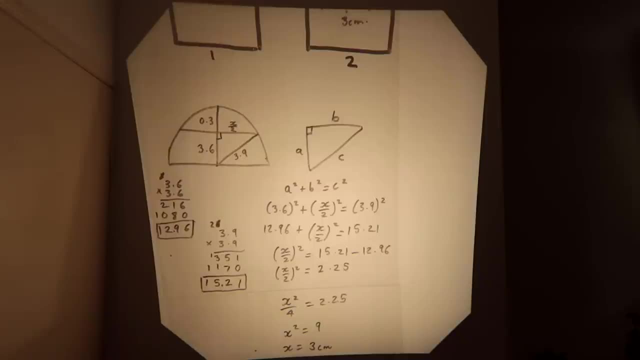 and so 3 will be the answer to this length in here. Now, I'm sorry to say, but we actually did it the slightly tedious way. There was something that we could have noticed which would have made these calculations redundant and the algebra a little bit easier, Perhaps, depending on how. 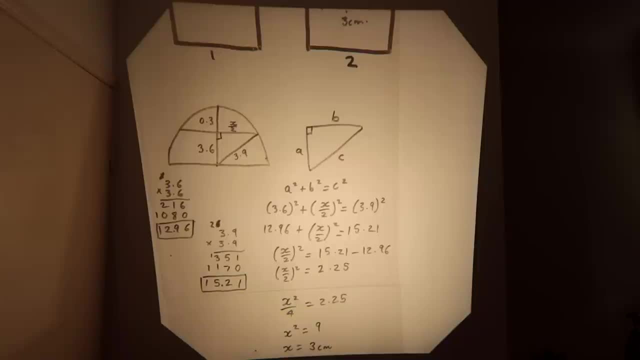 familiar you are with Pythagorean triples. Pythagorean triples are known sets of numbers that satisfy this. a squared plus b squared equals c squared. The smallest one is three, four and five. Let's take a look at a little bit of a visual proof of that. If I had a right angle triangle where one side is of length three, 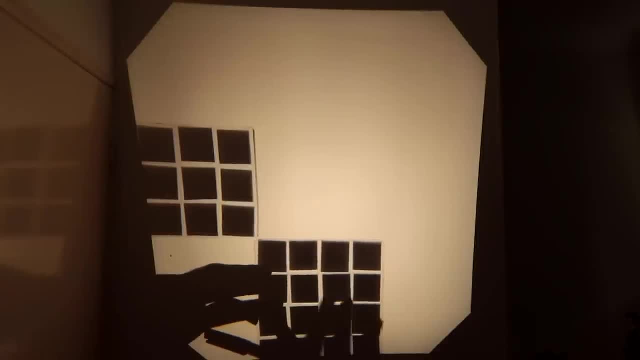 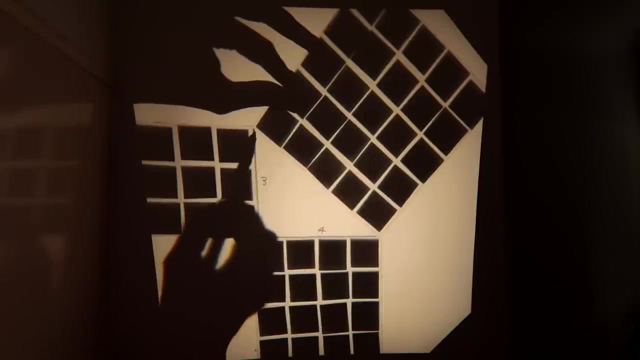 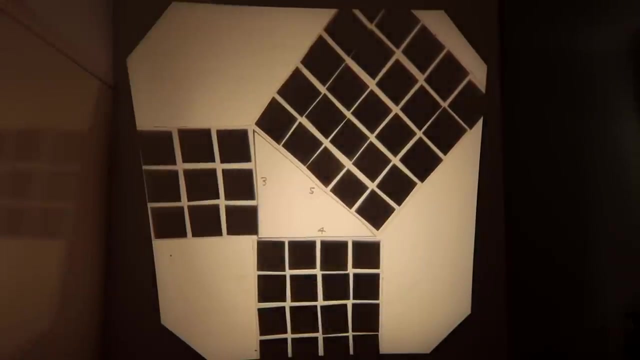 and the other side is of length four, then the length of the remaining longest side will be five squares. With the way that the light is projected up onto my wall, things up here look a little bit larger than things down here, but, believe me, I've tried to make all these individual squares the same size. 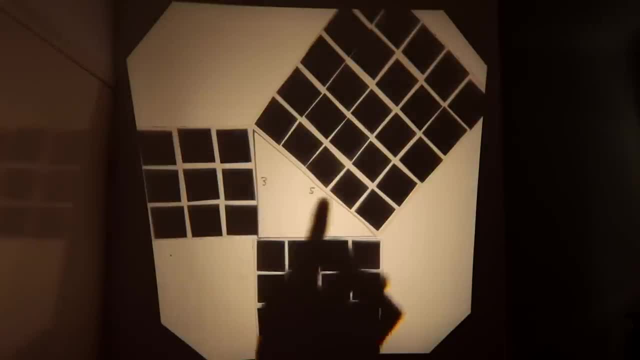 Each of these objects represents the side length squared. So three squared is this square. that's one, two, three, by one, two, three, a total of nine little squares. Four squared is 16, so there'll be 16 little squares here, and five squared is 25.. Pythagoras's theorem is saying: 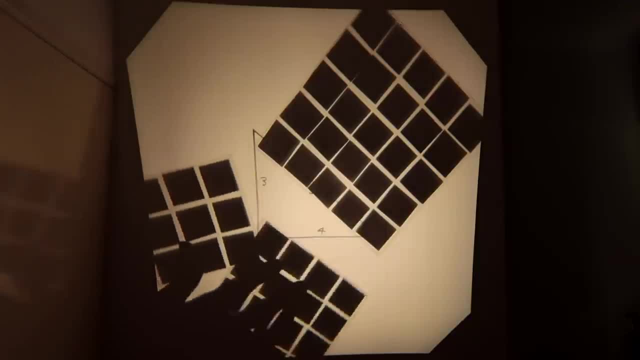 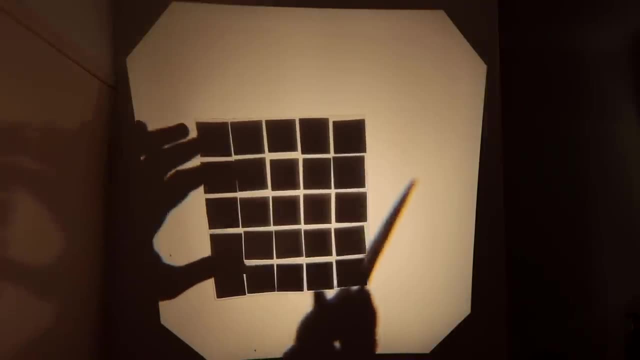 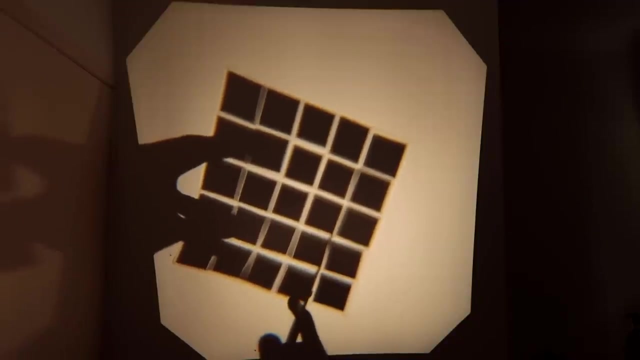 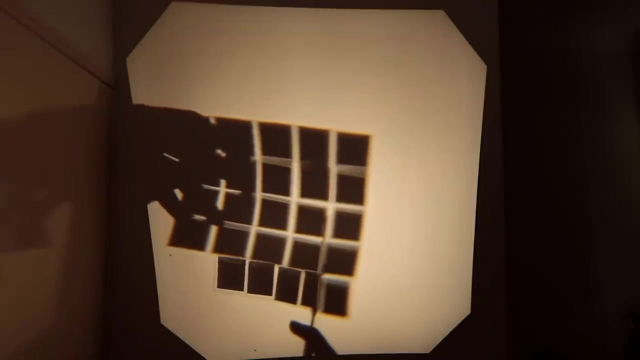 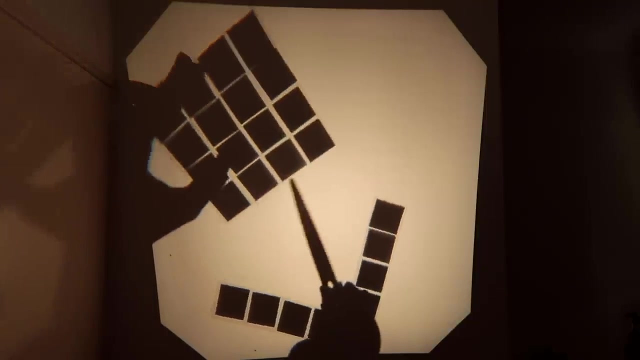 that the size of this should be the same as the sizes of these two added together. Here's our five squared, And I'm going to go at it with my scissors. From this I can cut out a four by four grid. Now I've got the four by four, but let's see if this little remaining. 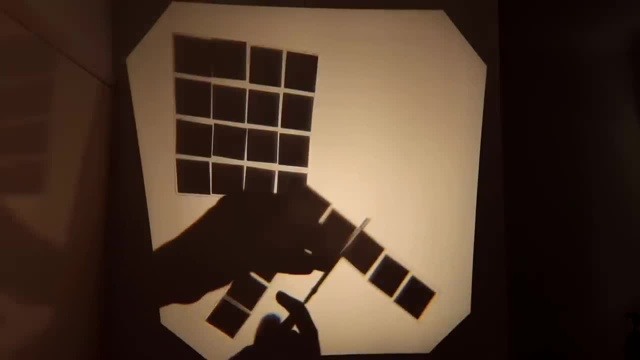 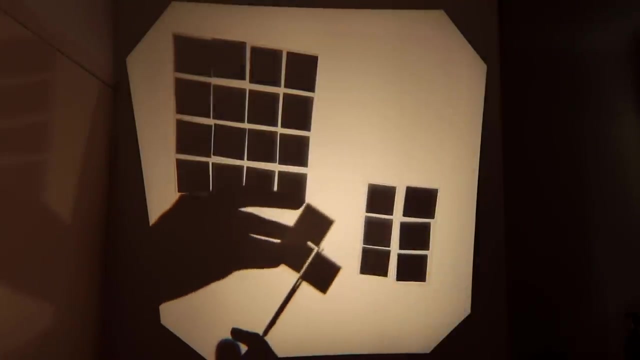 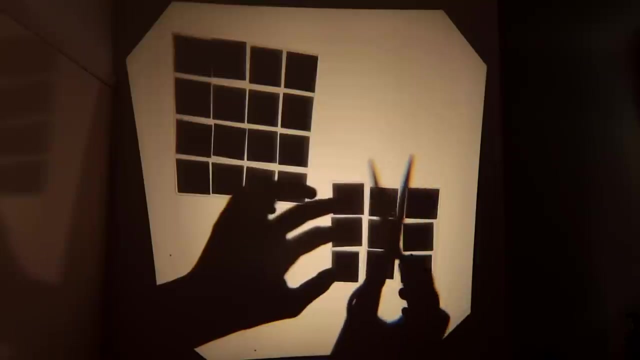 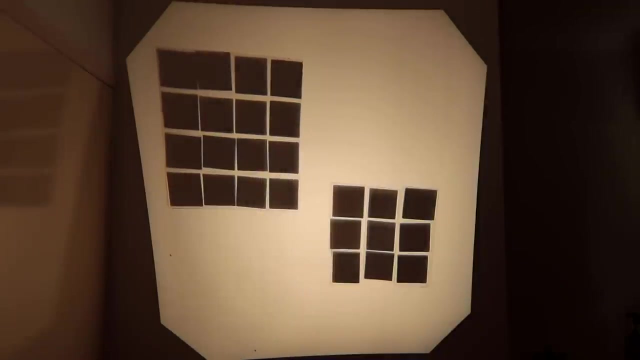 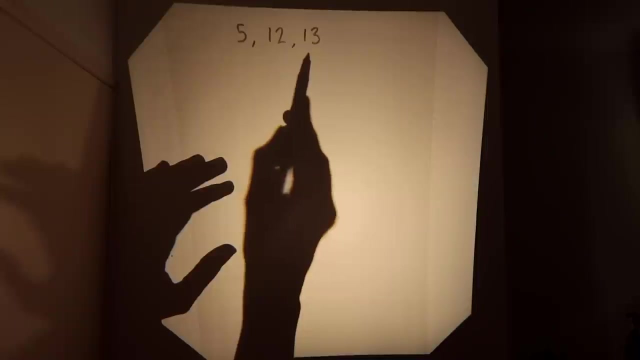 bit can be made into a three by three. And there we go. we can see our four squared and our three squared Popping out of that five squared with nothing left over. The next smallest Pythagorean triple is actually five, twelve and thirteen. 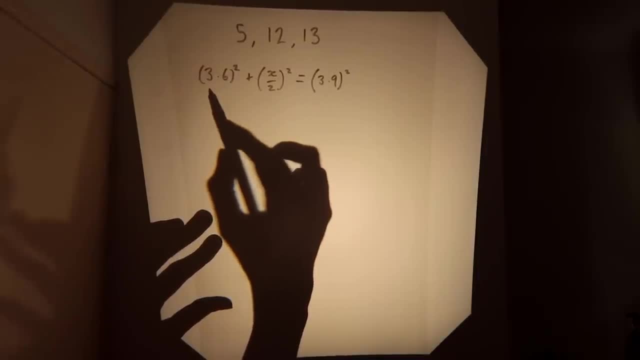 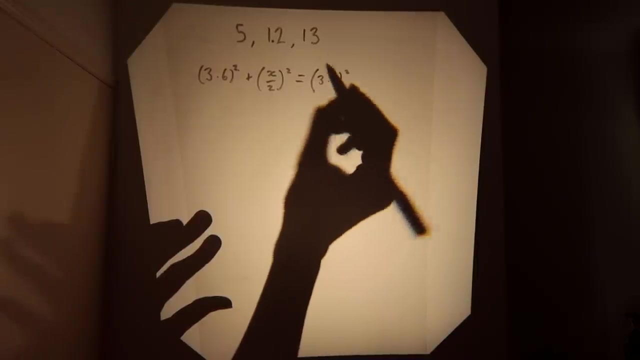 So when we were back at this stage, there is a chance that we could have noticed that 36 is 3 times 12, and so 3.6 is 3 times 1.2 and 3.9 is 3 times 1.3.. 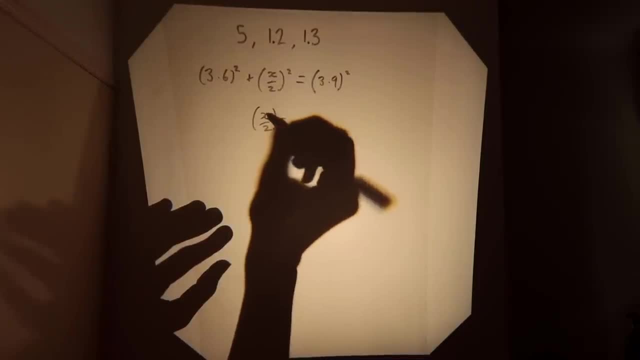 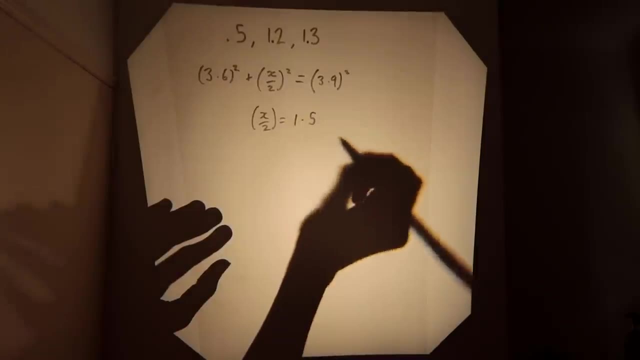 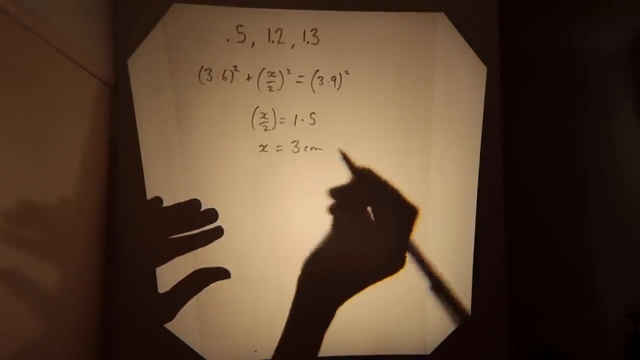 So, following our Pythagorean triple, x over 2 would have to be equal to 0.5 times 3, that's 1.5. So x would be equal to well. multiply by 2, that's 3 centimeters. A faster way to get the same solution that we had before. 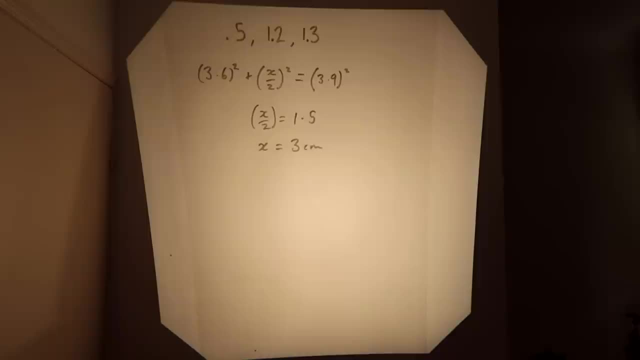 I don't know if you'll agree that it simplifies the math by much, but people have been using Pythagorean triples to simplify the math. I mean, they've been using Pythagorean triples to simplify their working for literally thousands of years. We've seen Pythagorean triples used on the world's oldest example of applied geometry. 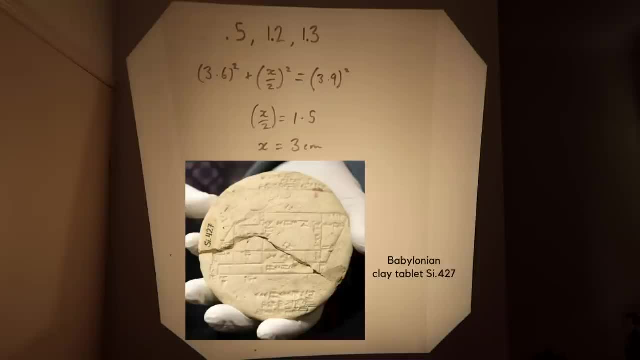 on a 3700 year old Babylonian clay tablet which laid out the division of land and boundaries of a field and used Pythagorean triples like 5,, 12, and 13, a thousand years before Pythagoras himself was even born. 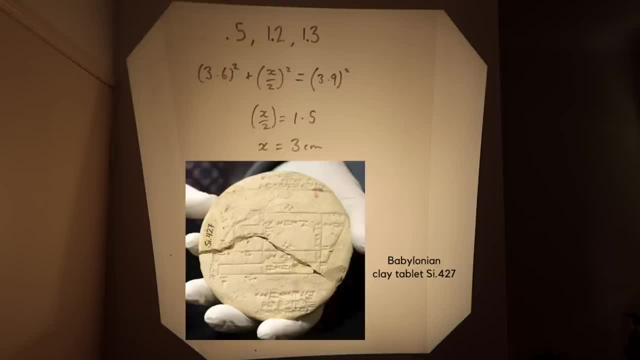 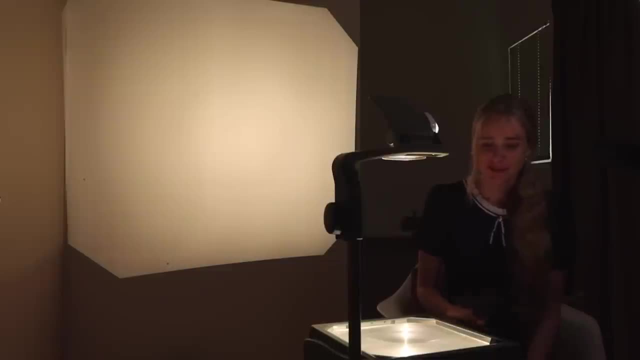 So Pythagoras himself was even born. So Pythagoras himself was even born. So Pythagoras himself was even born. Pyagoras wasn't the first person to invent this or to find these triples, but the theorem still holds his name. Our next stop is Australia. Now, this is an exam question from what is called the 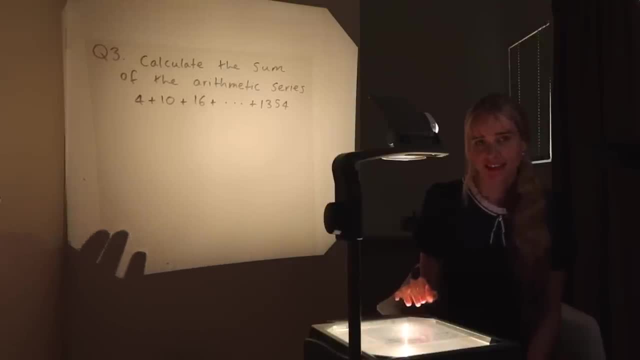 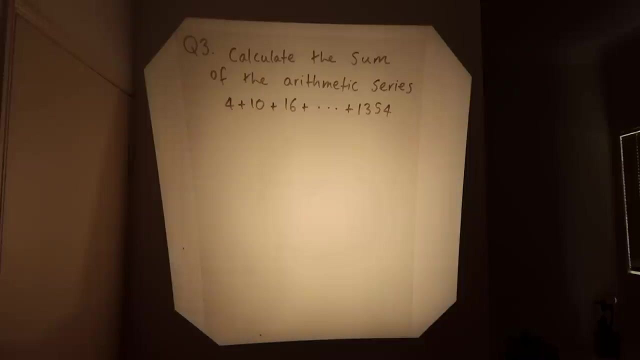 HSC advanced paper and that is something that would be sat by high school students in the Australian state of New South Wales. The question says: calculate the sum of the arithmetic series 4 plus 10 plus 16 plus dot, dot plus 1, 3, 5, 4.. An arithmetic sequence is a sequence of numbers. 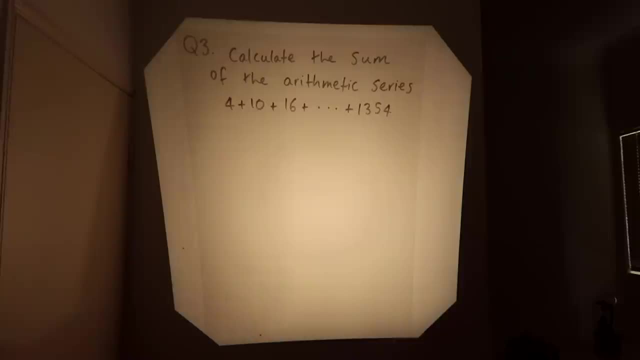 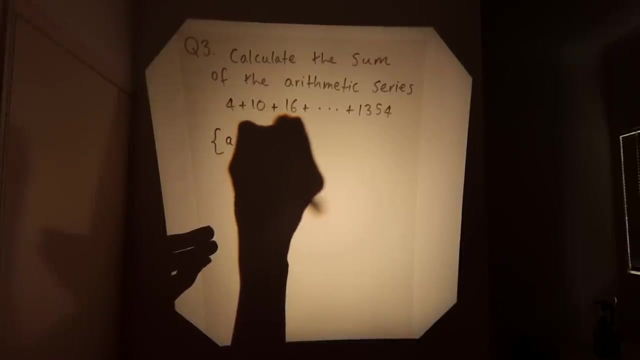 in which there is a constant difference between each term. so you're adding a constant amount every time. An arithmetic series is what it's called when you add all of these terms together. In general, if we called the first term of our sequence A, then our second term would be a plus d, where d is our difference and this one. 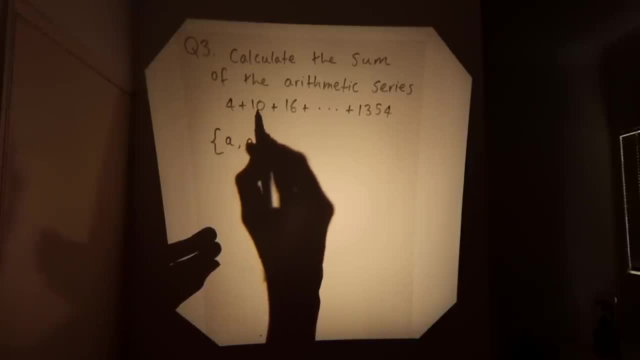 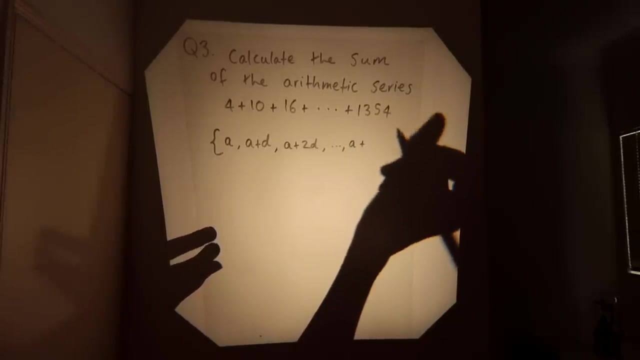 up here it looks like d would be equal to six. you've added six here and then again here, and so on. The third term of our sequence would be a plus 2d, then all the way up to our last term, which would be a plus. well, how many times have we? 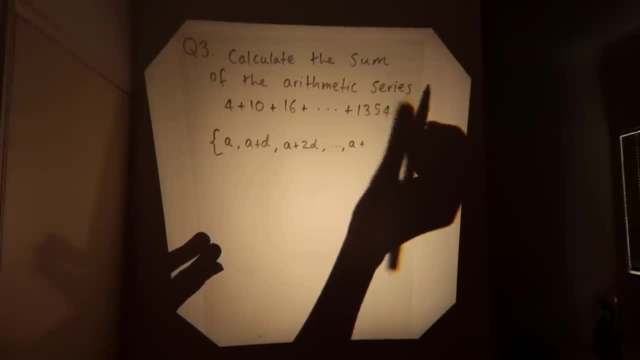 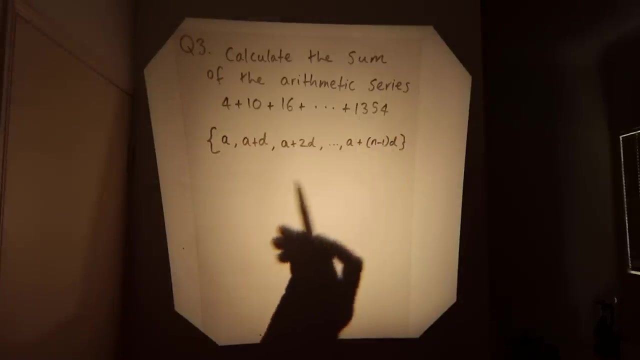 added d. If this is the nth term at the end and we started adding d from the second term onwards, then we would have added d n minus 1 times. If you already know the formula to find the sum of any arithmetic series, then you might. 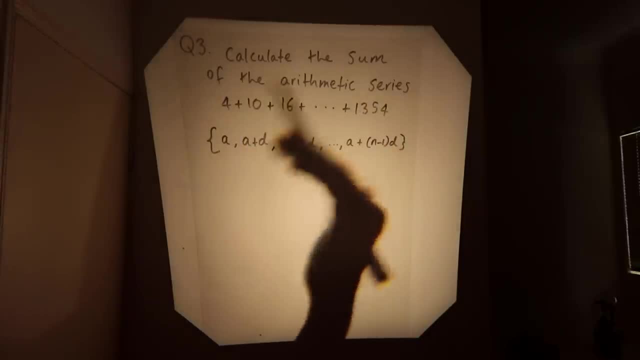 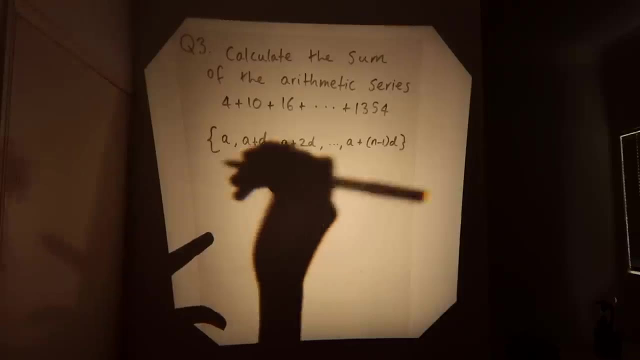 be able to look at this and plug it straight into that formula, but we're actually going to derive it. So how do you add up one of these things? Well, let's call the sum of our general series here S of n. We're going to add up each term starting with a, then a plus d. 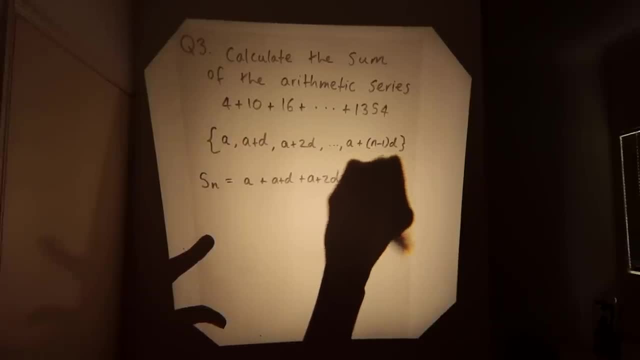 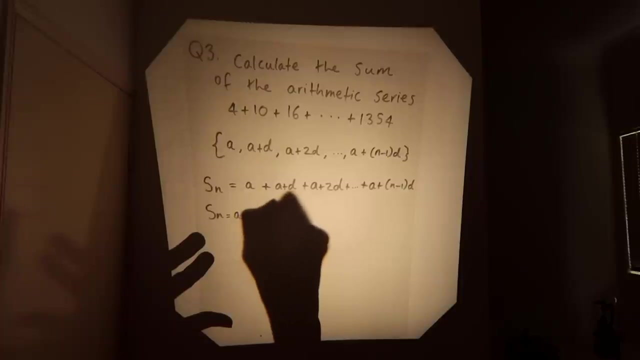 then a plus 2d, all the way to adding a plus n minus 1d. Now what we can do is write out the series again, but this time in reverse. We start with our last term, a plus n minus 1d, and then our second to last. 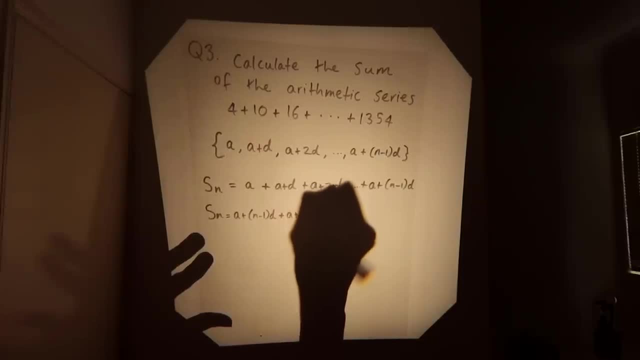 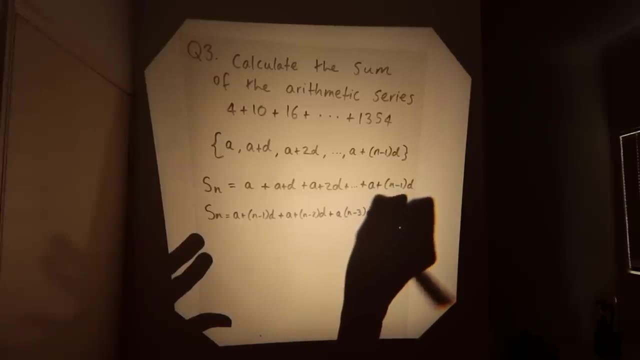 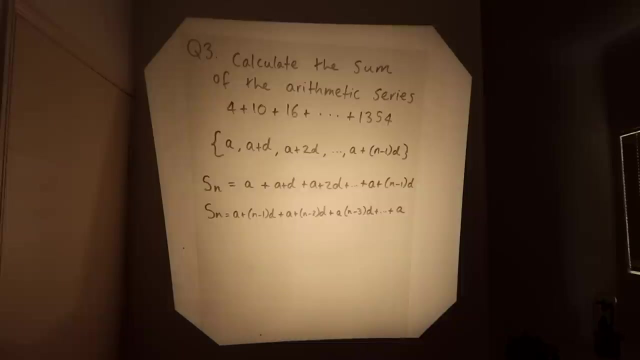 last term, which would be a plus n minus 2d, then a plus n minus 3d and, finishing with our first term, a. You often see mathematicians try this technique where they write out the series again, but backwards. that's because it allows them to do some kind of cool tricks. 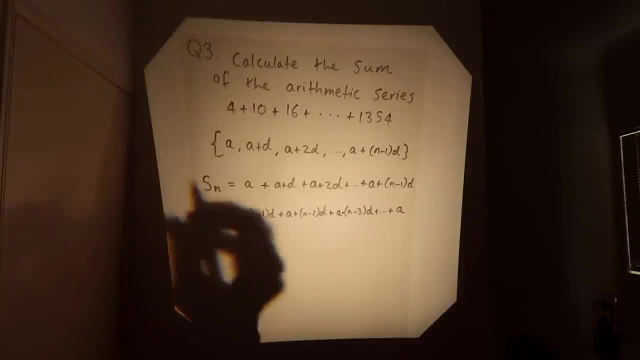 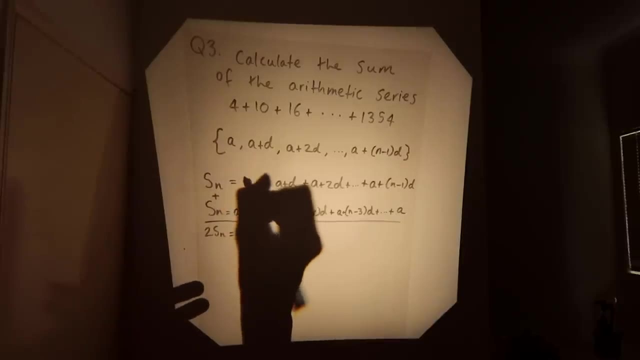 one is to add these two series together. we add s of n to itself. doing that, we would get two s of n's. The first term of that would be a plus a plus n minus 1 d. Well, what is that? a plus a is 2a plus n minus 1. 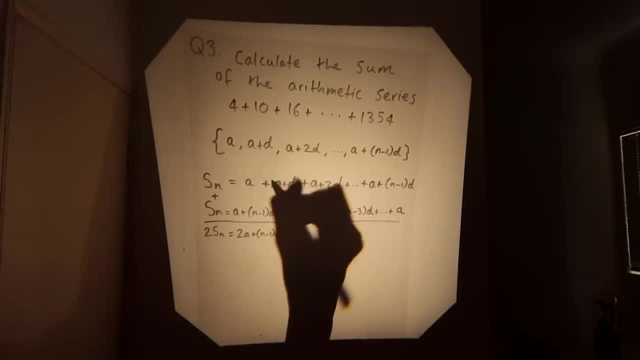 d. The next term is a plus d plus a, plus n minus d- 2d, and that might look pretty different. but actually what do we have? An a here and an a here, 2a plus. well, we have n minus 2d plus an. 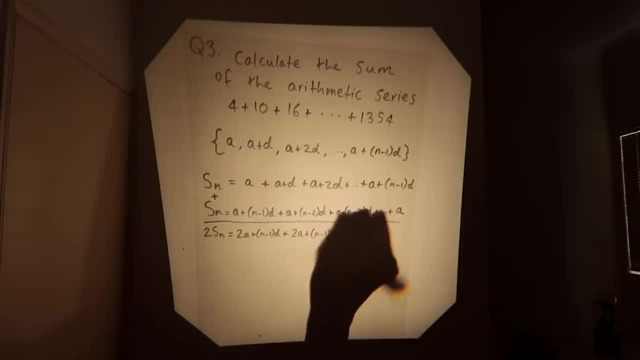 extra d, that's actually n minus 1 d, and in fact every term in here gives you that same result. I'm going to run out of room on my transparency, but a plus 2d plus a plus n minus 3d is also equal to 2a. 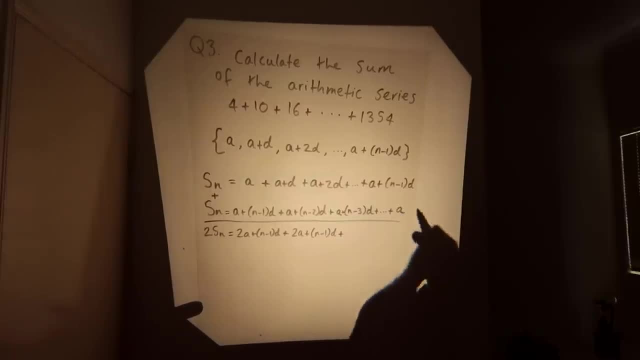 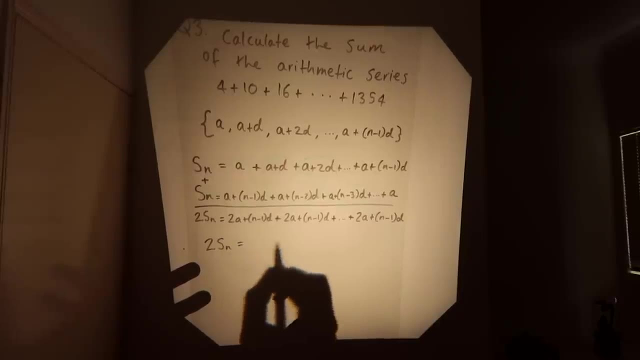 2a plus n minus 1 d, and you can see it pretty obviously with our last term too. So in total we have that 2 times s of n is equal to this term. 2a plus n minus 1 d, repeated for however many terms we have. 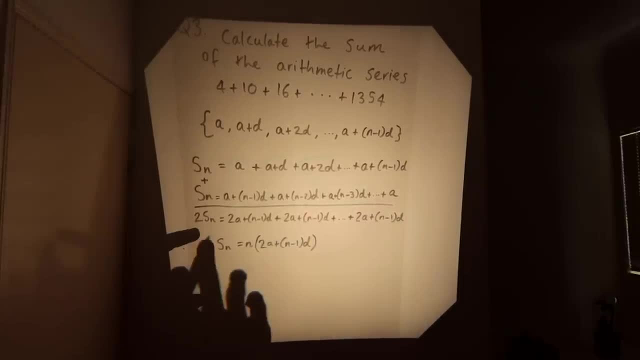 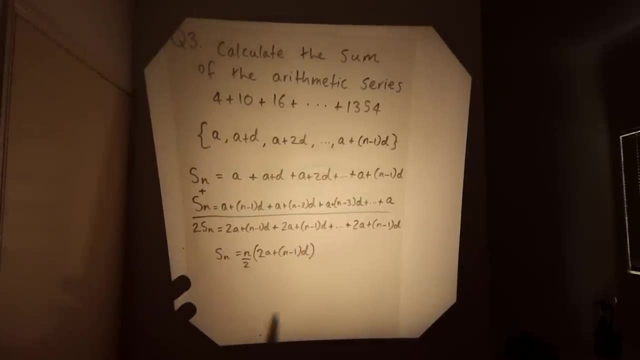 so repeated n times To get rid of the 2 and get us the expression just for one series. we can do n over 2 and we can simplify it just a little bit more. If we look back to our sequence, the last term is always a plus n minus 1 d, and we kind of see most of that in here. 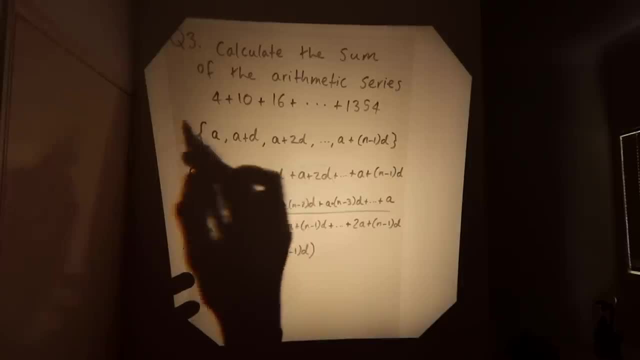 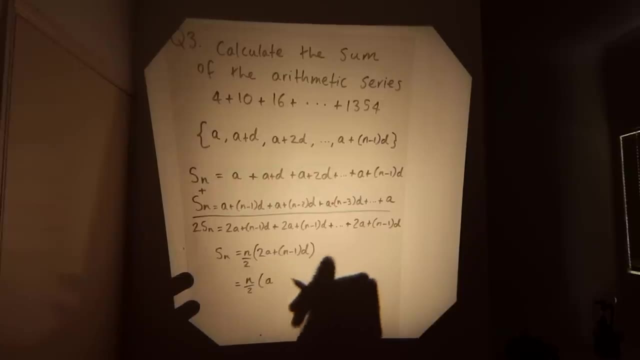 although we have an extra a and well, a is always the first term, So this can also be written as n over 2 a, which is the first term plus the last term. maybe we can call that l. Now that is a derivation of what will. 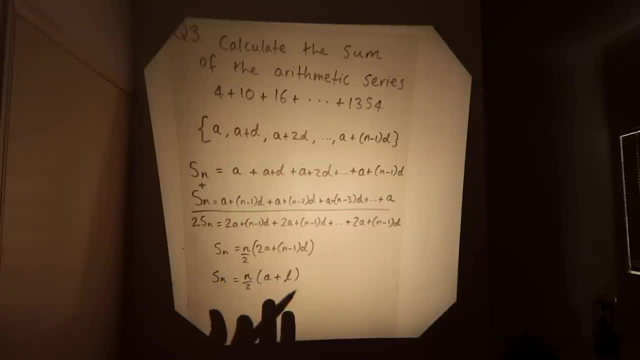 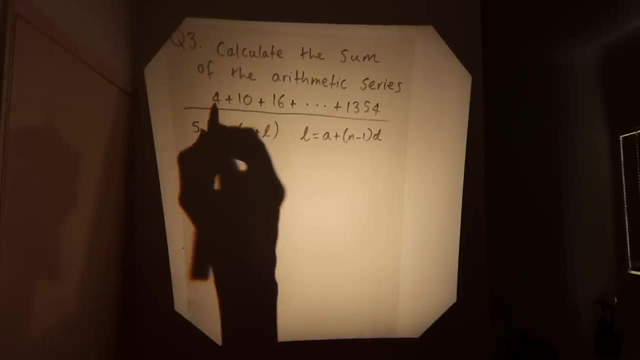 always be the sum of an arithmetic series. So let's get to working out our problem. We have what we've derived just here and we know that. well, there's a constant difference of six between each of our terms. so d for us is going to be equal to six. 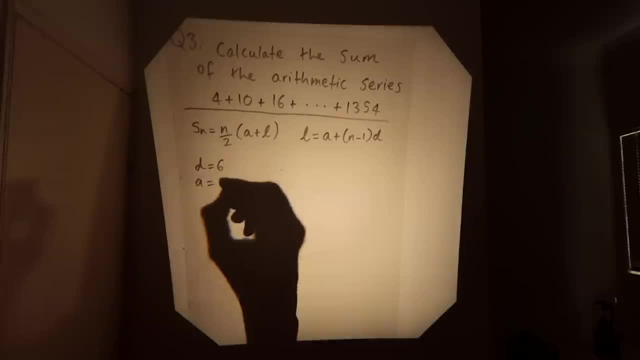 Our very first term, a, is equal to four, and our very last term, l, is equal to one, three, five, four. We don't, however, know our value of n. They haven't told us how many terms there are, so we can't jump straight into using. 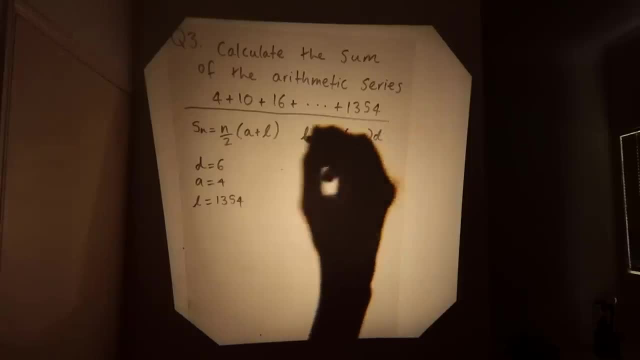 this one. Instead, let's put what we know into this formula here for our last term. If one, three, five, four is equal to four plus n minus one times six, then subtracting the four and dividing by six, we have one, three, five o divided by six is equal to n minus one. 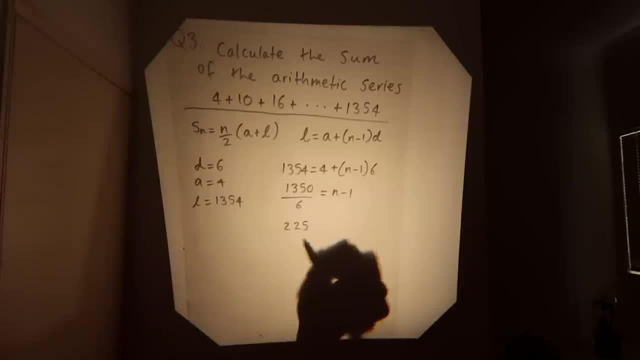 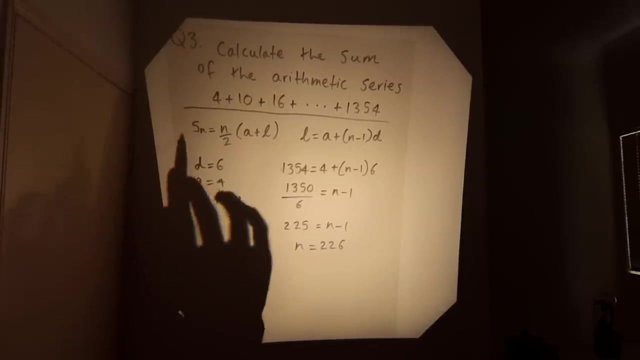 That will be two, two, five. I think you might be allowed a calculator for this exam. this is the Australian one is equal to n minus one, and so n is one plus this. n is equal to two, two, six. Now we have n and all that we. 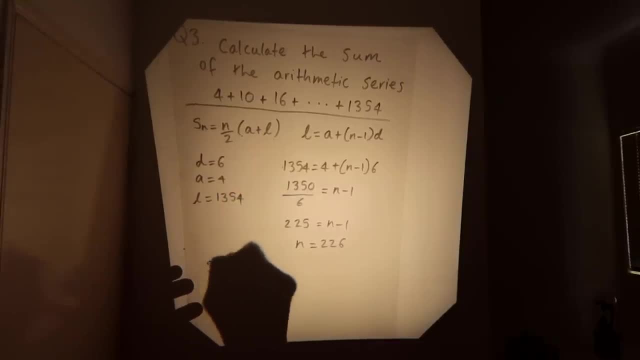 need to calculate. the sum of all the terms is equal to one, three, five, o divided by six sum. so s of n is equal to two, two, six over two, the first term plus the last term. Well, if we plug all this into the calculator, we end up with: 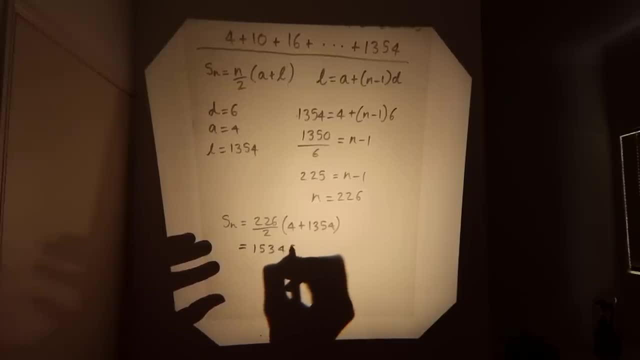 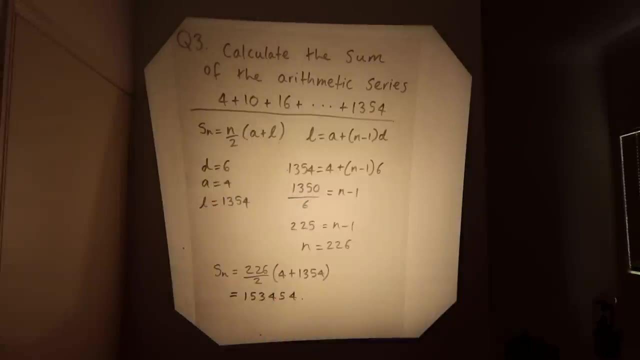 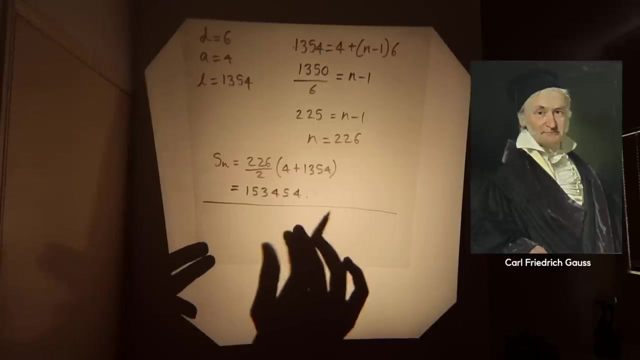 one, five, three, four, five, four as our answer. Well, who would have guessed? that's what it is. adding up all that, This question reminds me of a little story that goes around about the mathematician Carl Gauss. He's known as perhaps one of the greatest. 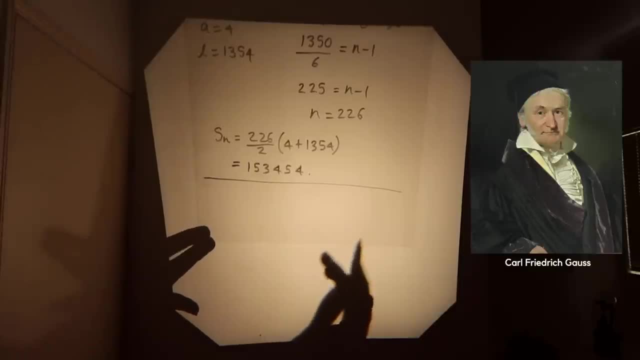 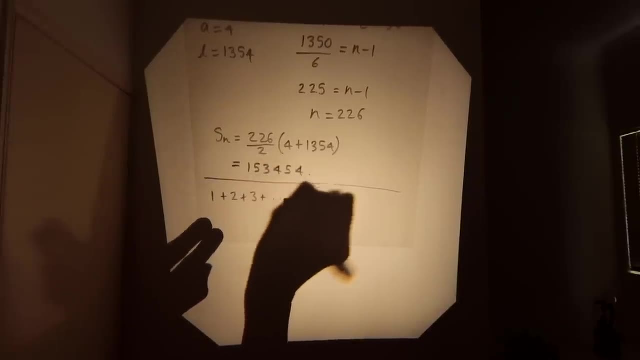 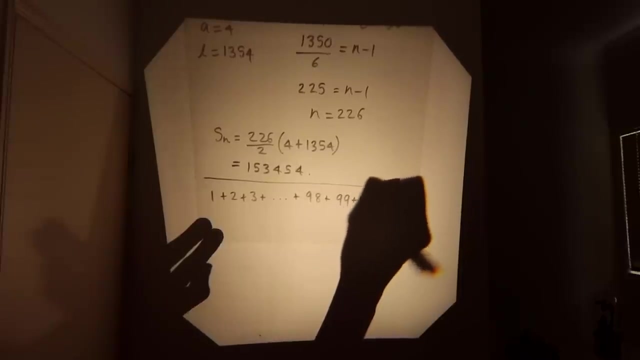 mathematicians, and this is a story from the time when he was at school. Apparently, Gauss's teacher wanted a bit of peace and quiet, so he asked the class to add up all the numbers between one and a hundred. As the other students set about adding it all up very slowly and carefully, 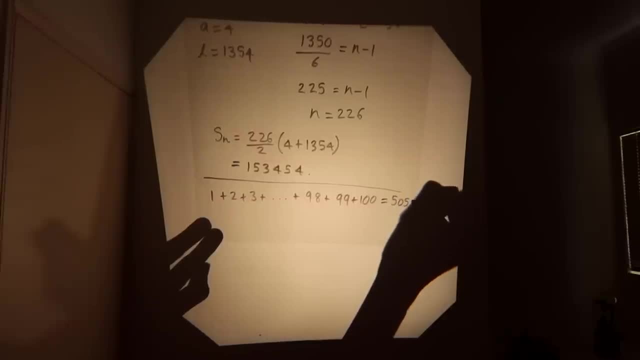 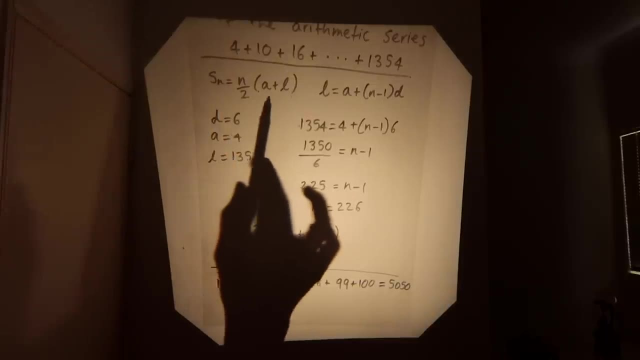 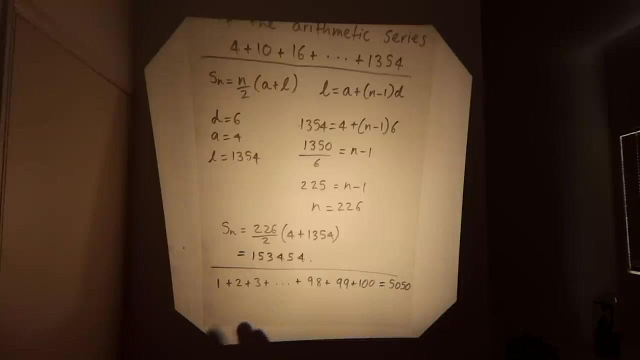 Gauss almost immediately wrote down the correct answer, which was five thousand and fifty. Gauss could perhaps see a formula similar to this one and applied it to the problem. He's said to have imagined it as folding up these numbers in half and then adding up the pairs, such as one and a hundred and two and ninety. 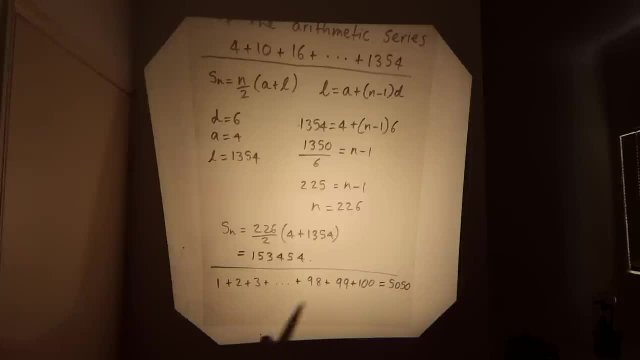 nine, That would be fifty pairs of a hundred and one giving the answer, or, expressed as a formula, the first and last term times n divided by two. Now, this anecdote tends to make the other students in the class sound pretty unintelligent, as if they would add up. 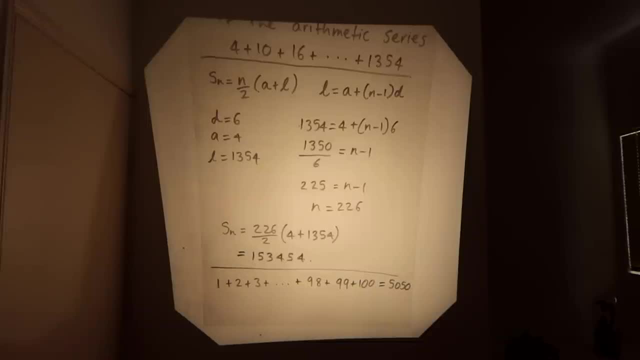 one plus two plus three and do every single step in order. but i challenge you to imagine doing this for yourself, even if you knew nothing about math or sequences and series and these formulas and tricks. As you go through the numbers, you can't help but see some patterns. In fact, it almost seems difficult to do. 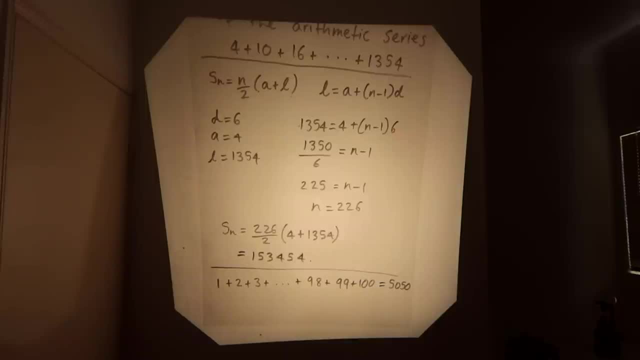 it in the hardest way. You'd see that in adding up the numbers between 10 and 19, you'd get the same sum as adding up the numbers lower than that, just with an extra 10 sets of 10.. So just because you're not, 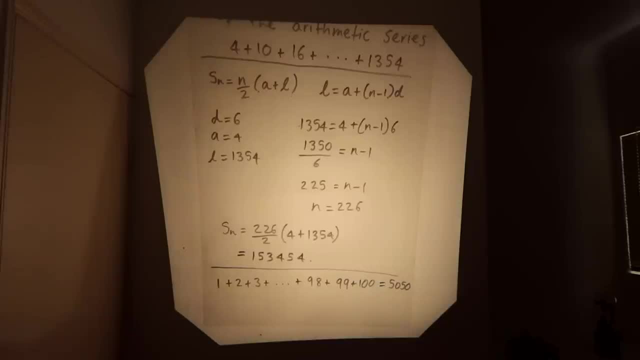 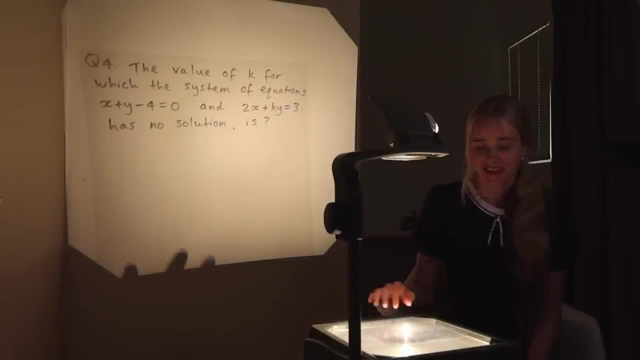 Gauss, answering it in a few seconds doesn't mean there aren't lots of ways to solve a problem like this. This next question is from India. Now, often, when i've spoken about Indian exams on my channel before, i've spoken about things like the JEE. 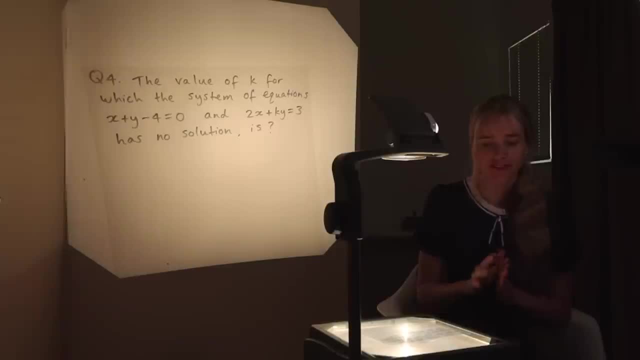 which is a super specialized engineering focused, really difficult paper for university entrance. but this question here is from the CBSE exams and in fact the standard mathematics exam for grade 10.. Now this isn't even the most advanced paper. we could have gone to grade 11 or 12. 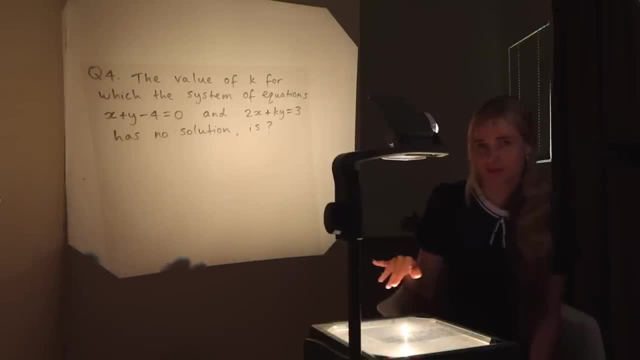 but i found that picking the grade 10 one brought it a little bit more in line with some of the other problems i've picked and made it a little bit easier, you know, For this video where i don't want to stress you out too much. 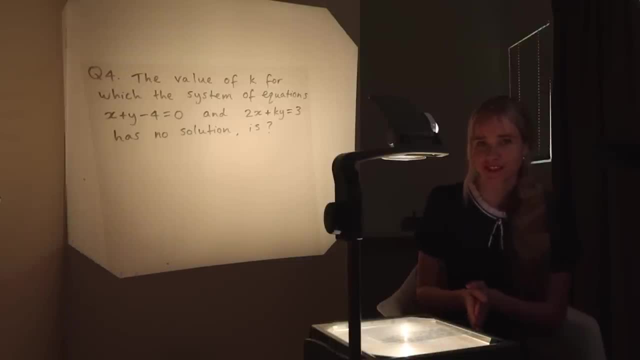 so the the user. CBSE exam papers from India are more standard, sort of, given to everyone rather than just those people who want to specialize in engineering. So let's have a look at the problem. It says the value of k, for which the system of equations. 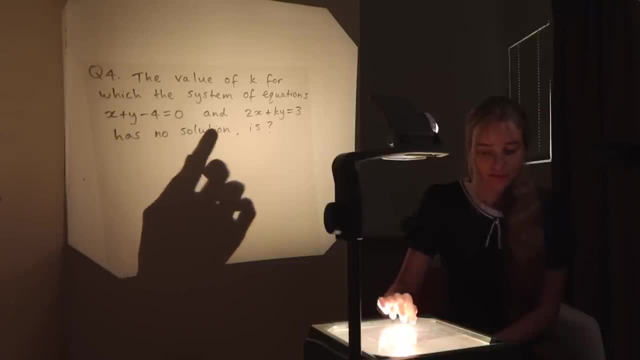 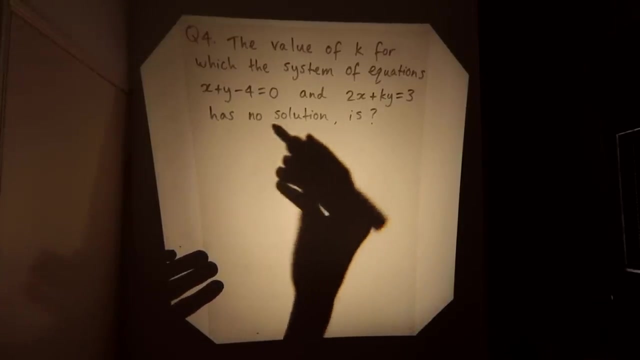 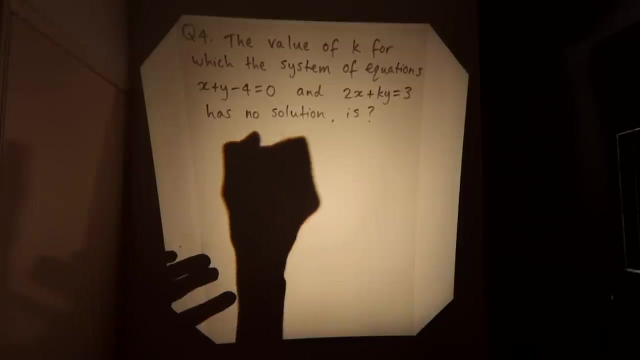 x plus y minus 4 equals 0 and 2x plus ky equals 3, has no solution. is what? All right? equations like these represent straight lines, and when we're talking about solutions of systems of equations like this, we can imagine where the straight lines might intersect. 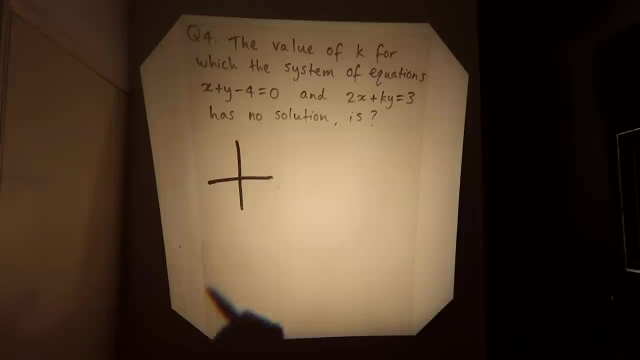 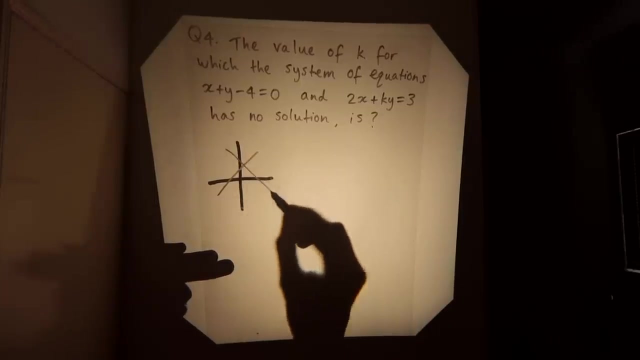 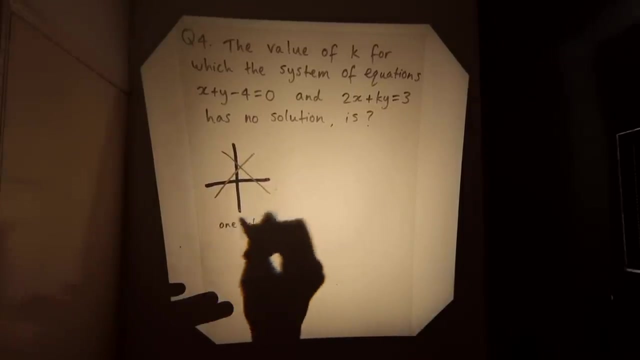 So if we have an x- y axis like this, then in the case where, for example, one line might go like this, the other might go like this, we have one place where the lines intersect, and that would represent one solution. We also refer to this situation as being: 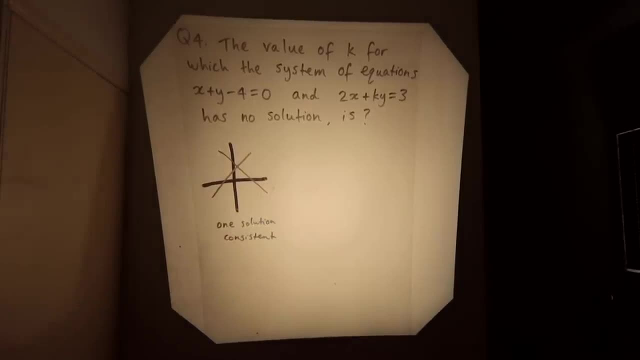 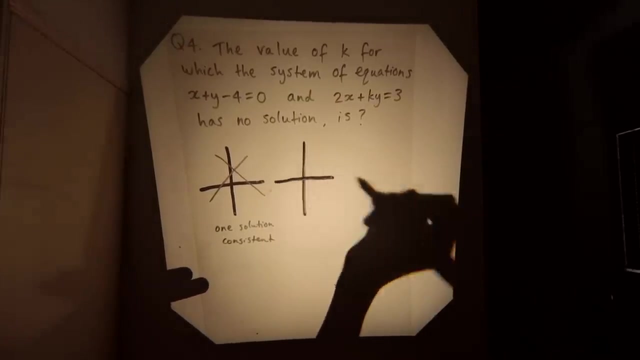 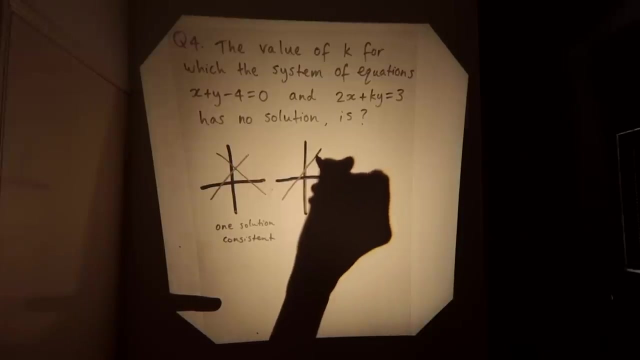 consistent. Let's try another possibility: If we have one line and then another line exactly over the top of it, so that you can barely even tell them apart, well, we're going to have infinite solutions because since these lines are perfectly over the top of each other, 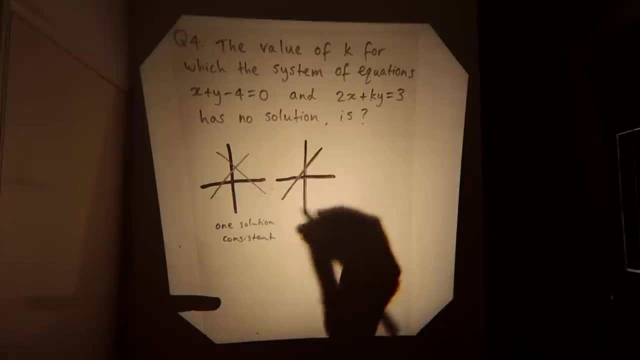 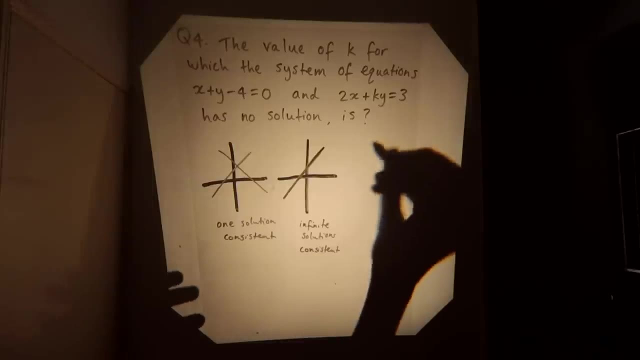 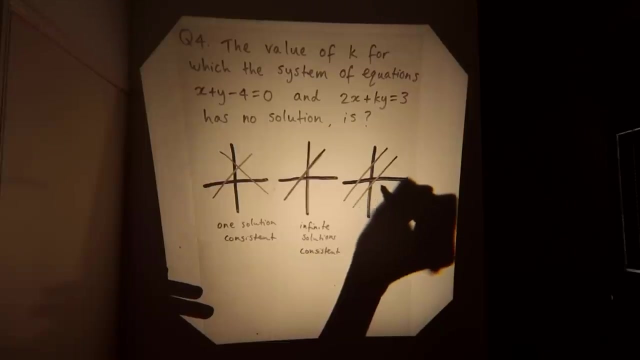 there are infinitely many places where they meet. the situation is also referred to as consistent. And there's one last possibility to consider, and that is in the case where our two lines, one here and one here, are parallel to each other. they're like train tracks, perfectly. 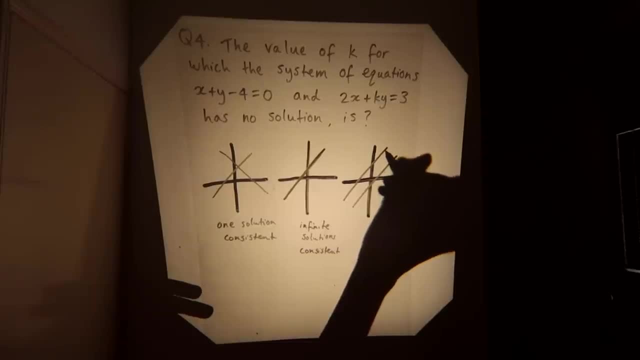 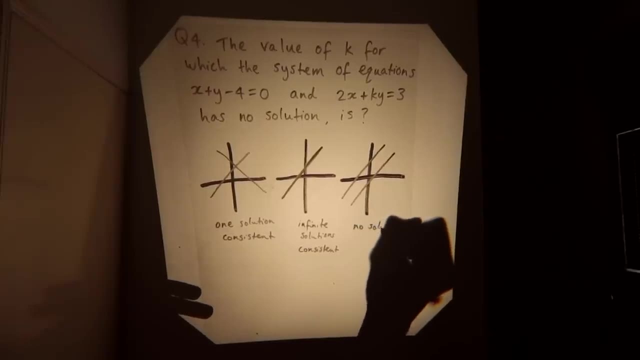 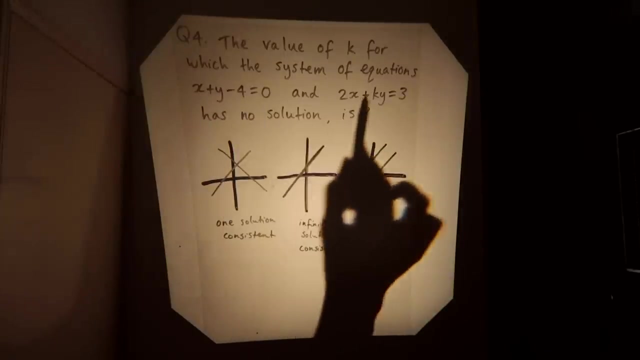 parallel and they're never getting closer or further away. they're always staying the same distance apart. in this case, there will be no solutions. the situation is referred to as inconsistent, so in our question we're asked where these two straight lines have no solution. so really we're asked how we can ensure that these lines will be. 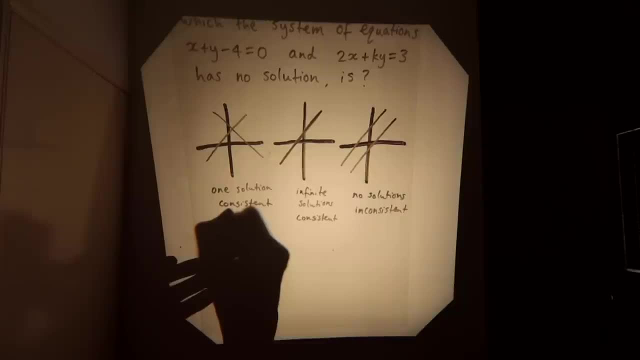 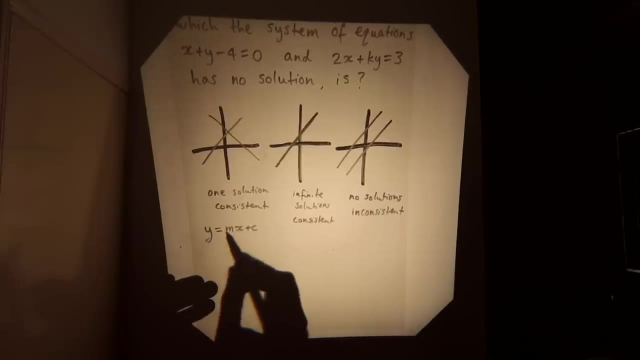 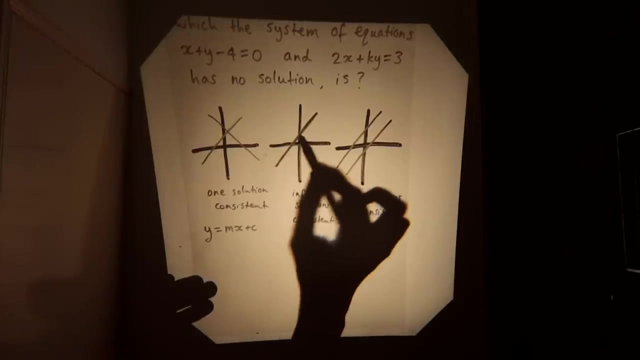 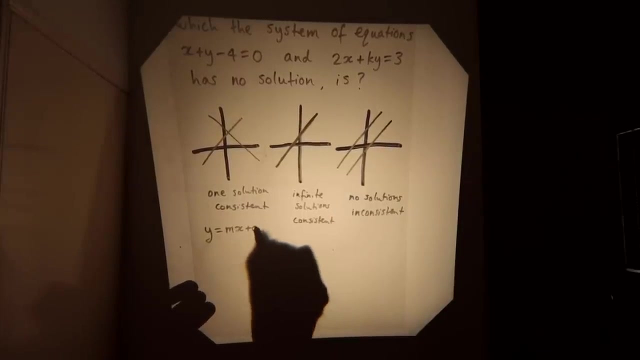 parallel. we often see straight lines written in this format: y equals mx plus c. this is the intercept format and here m represents the slope of the line and c represents the y-intercept. so where it cuts the y-axis For two lines to be parallel, they would differ only in the y-intercept, so they would have the same gradient but just shifted up. 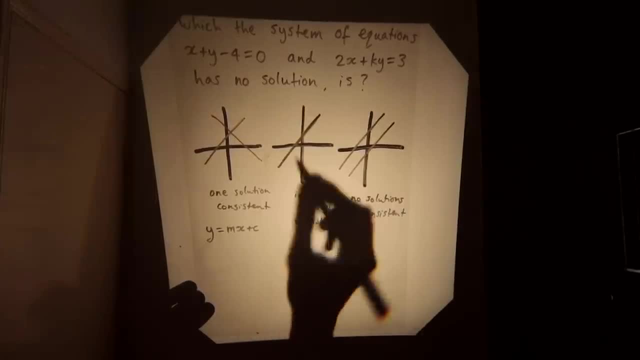 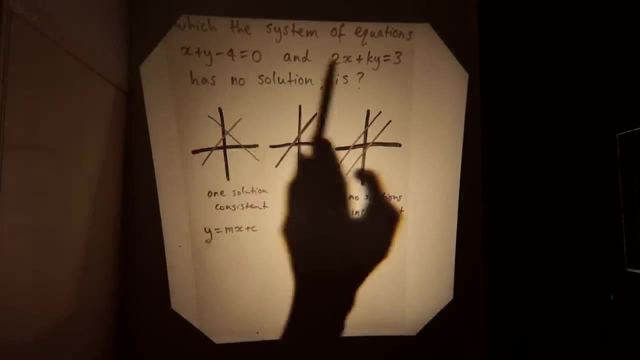 or down by some different amount. c. If c was the same and the gradient was the same, well, they'd be on top of each other. So one way to solve this is to rearrange both these equations into this form and see what you can do to make sure that m is the same for both lines but that c is different. 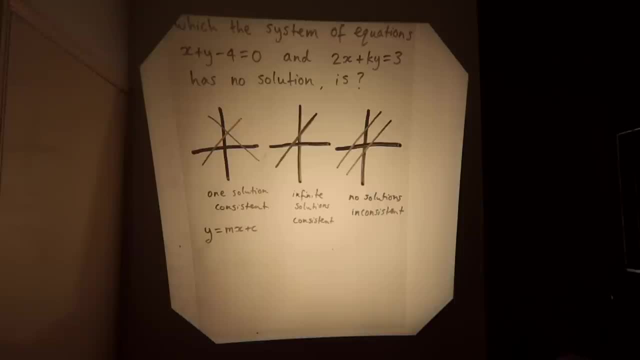 But this is a question on an Indian exam and they love to find tricks where you can solve these questions almost instantly. Sometimes that involves memorizing a lot of seemingly random little formulas and equations to solve these quickly and maybe, in the extreme time pressure of exams like this, maybe even rearranging it into this. 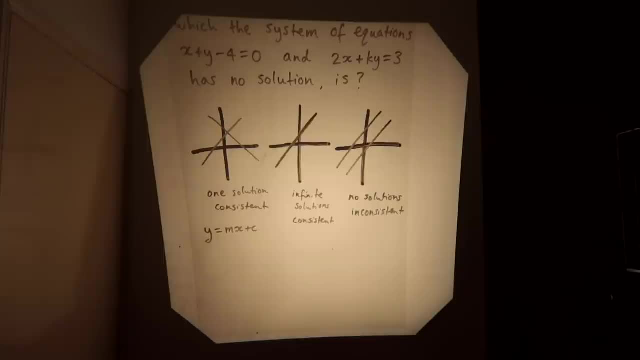 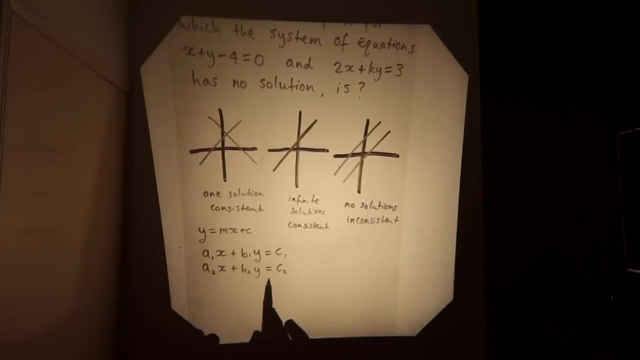 This form is way too slow, So let's see where a shortcut might come from. In general for simultaneous equations in this form, ax plus by is equal to c. Often we can solve the equation by adding these two together and hopefully in a way that cancels out one of our variables. 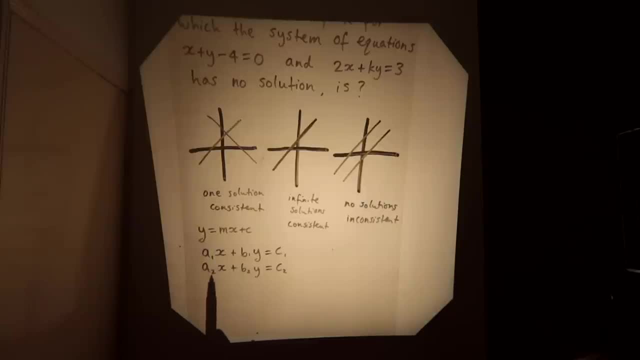 For example, if a1 was 1 and a2 was minus 1, then adding these two together would remove the variable and you would be able to solve for y If a1 and a2 or b1 and b2 aren't already the same magnitude. 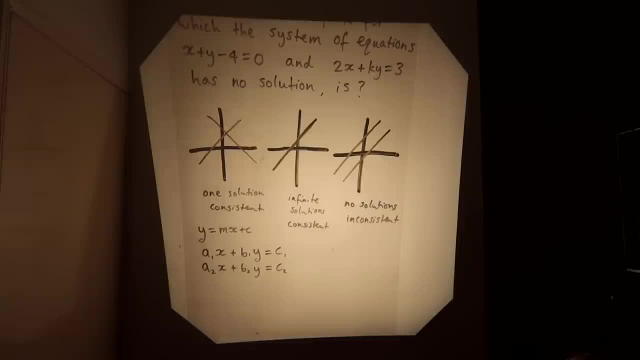 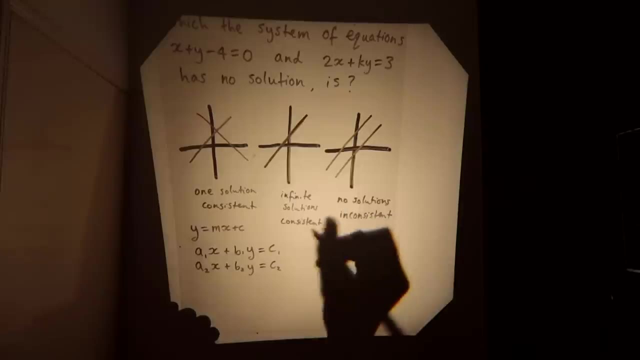 we can multiply them by some constant to make sure that they are. We just have to make sure to multiply every term by that same constant. For us, our equations can be written as: x plus y is equal to 4 and 2x plus ky. 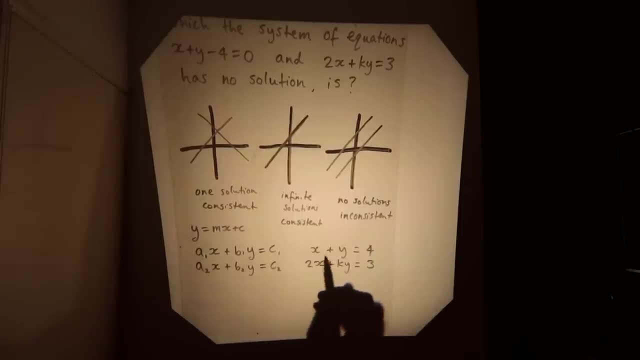 is equal to 3.. If we multiply the entire top equation by minus 2, then adding these together, we would see the x variables disappear. We would have minus 2x. minus 2y is equal to minus 8.. That's all fine, because we did it to every single term. so it's the same equation Adding these up, we. 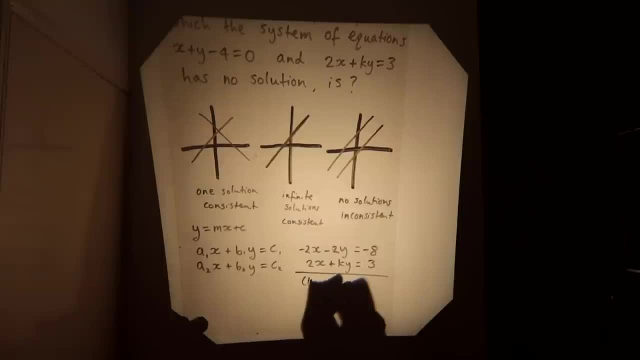 have 0x, then 2x minus 2y is equal to minus 8.. That's all fine, because we did it to every single term, so it's the same equation. Adding these up, we have 0x, then k minus 2, y being equal to minus 5.. Now we don't know what k is, but that's the thing we're trying. 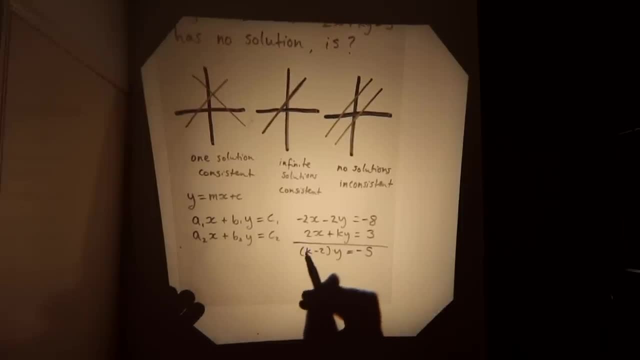 to find. Let's have a think about it. If k was any value except for 2, this would look like a normal equation. We'd have something: times y is equal to minus 5.. We could find that y is equal to minus 5 divided by whatever this value is. That would represent a consistent set of equations. 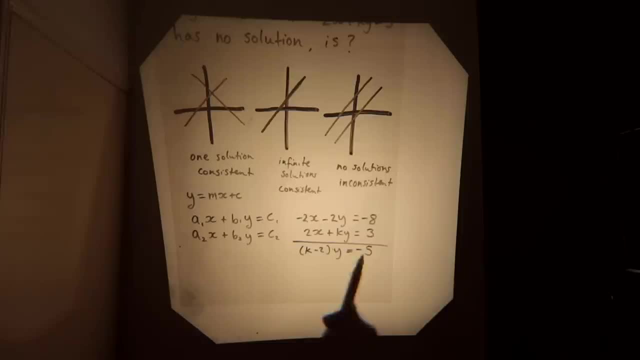 one where there is one solution. but what if it gets weird? what if k is equal to two? we'd have two minus two, that's zero. zero times y is still zero, and we would end up with zero is equal to minus five, that is, if k is equal to two. now, believe it or not, this is actually what we want. 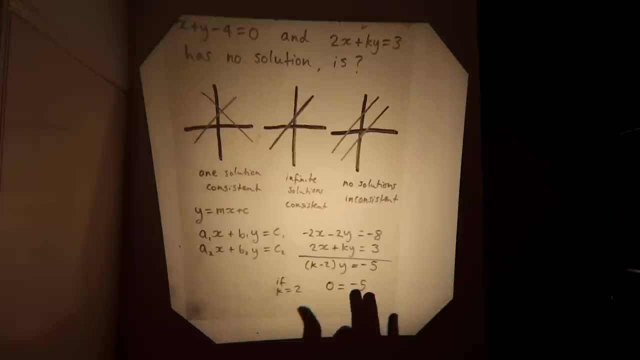 seeing something like zero is equal to minus five. well, that is inconsistent. there is no solution to this, because, well, think of it like this: what values of x and y result in zero being equal to minus five? well, none. there are no values of x and y that ever make this true. this is inconsistent. 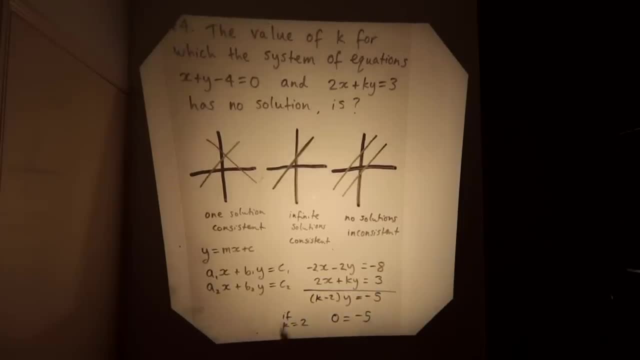 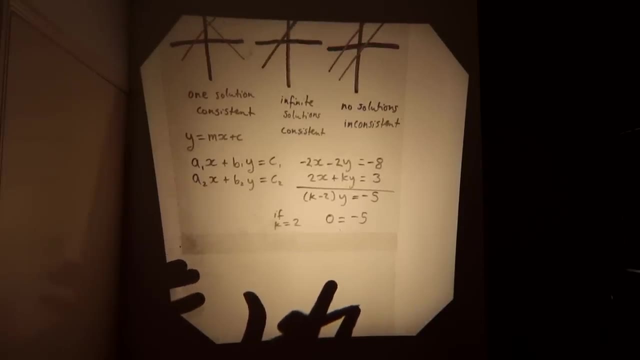 in the truest sense of the word. so the answer to the problem is actually: k is equal to two, and if you're an indian student studying for an exam, you probably already know a shortcut way to think about this. it is to say that for no solutions. we want to ensure that. 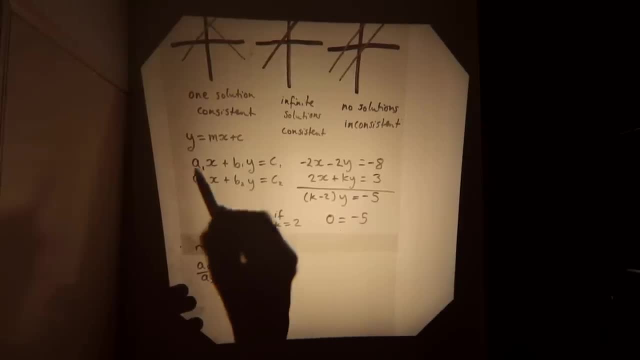 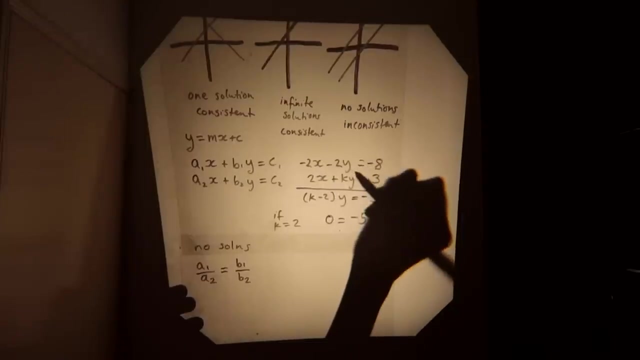 the ratio a1 over a2. that's these values here we want to ensure that is equal to the ratio of b1 over b2 basically means that when you decide to multiply it by that constant minus two, that we cancel both our x's and our y's, because these ratios are equal to each other. but we do. 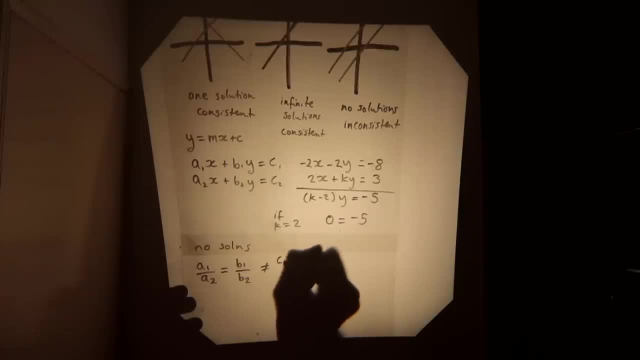 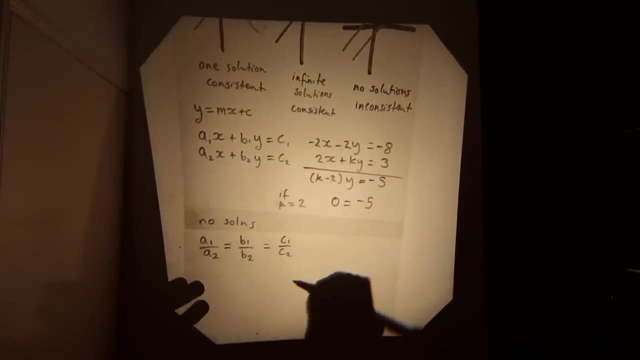 not want both of those to be equal to the ratio of the constants c1 over c2. that is the shortcut way to find the answer to this problem. so if they had have also been equal to c1 over c2, well, in that case the constants would have also cancelled out and we would have been left with. zero is equal to. 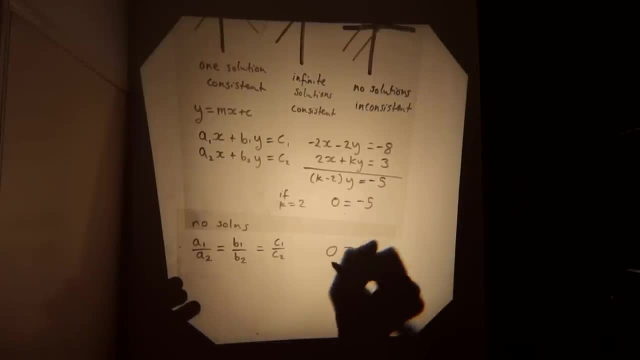 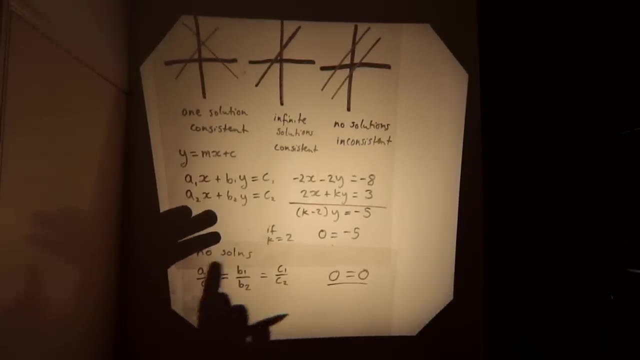 zero, that doesn't mean that we can't find the answer to this problem. so we can't find the answer to this problem so it doesn't represent no solutions. in fact, this is always true. zero is always equal to zero. so if this is the ratio between all the coefficients, you actually get. 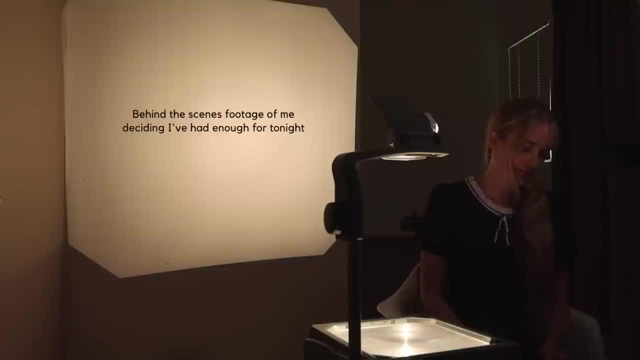 infinite solutions now. i also had questions prepared here from the uk's gcse and from the american sat exams. but i'm looking at my camera- it's been filming for a long time. looking at my mic- it's about to run out of batteries and i'm starting to feel like maybe i've done enough already, so perhaps i'll save those extra. 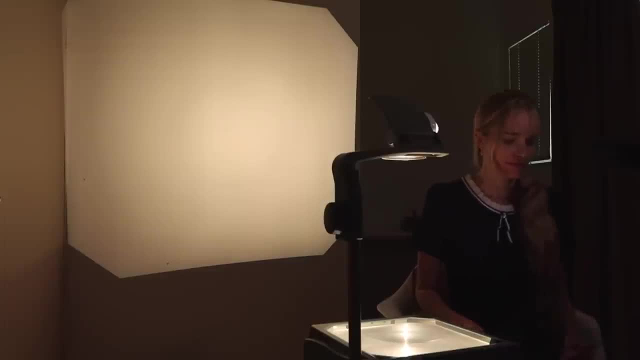 two questions for a part two, or if anyone enjoyed this video or made it to the end, let me know and i'll know to keep them for later. thanks so much for watching this video. i know it's been a little bit different. it's been a little bit of a risk for me to do. if you've been listening, to try and 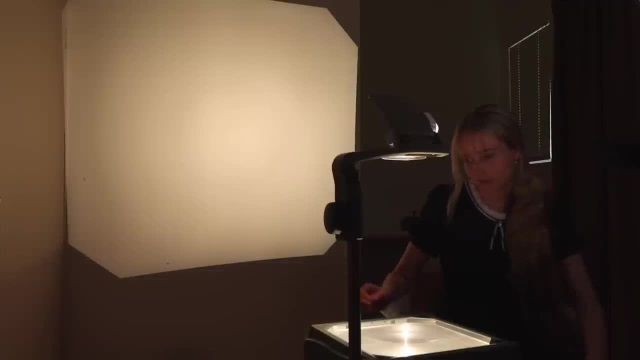 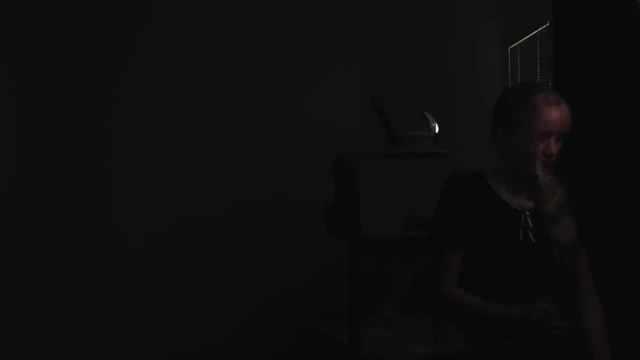 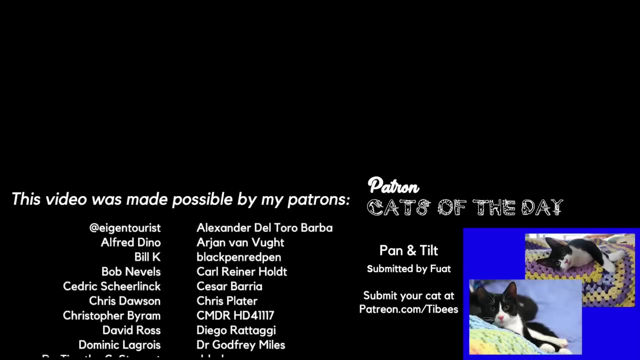 fall asleep, then good night, and if you've been watching to relax or unwind, i hope you've had a good day and i hope that the rest of your day is positive and not too stressful, that you get some good stuff done. thanks, as always, to my patreon supporters for making my videos possible and a 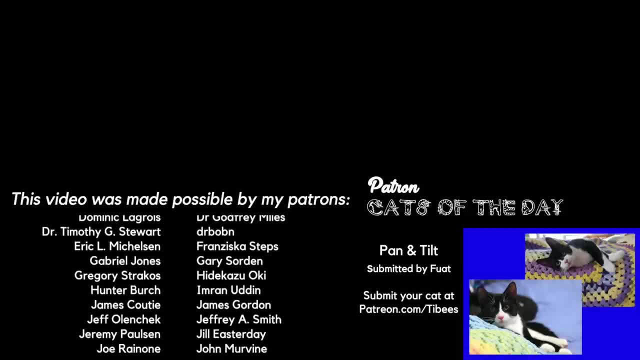 special shout out to today's patreon cats of the day, who are very astronomically named pan and tilt. 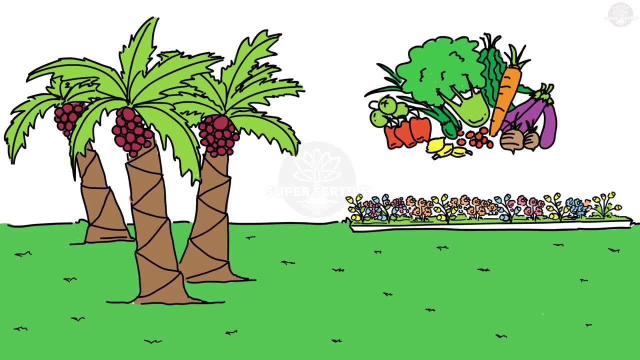 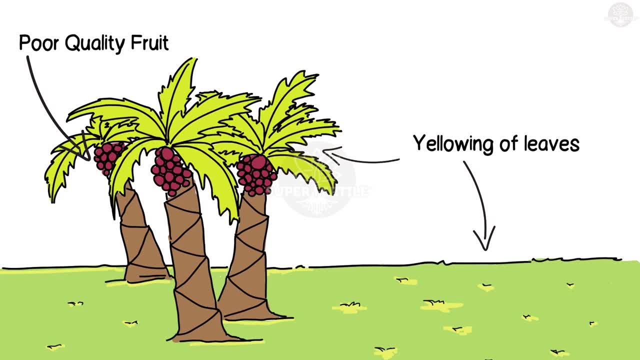 When you are looking after your plants, what you don't see is as important as what you do see. You notice your plants do not grow well, despite giving them the right nutrients. Why? That depends on your soil's pH. Soil pH is the measure of the acidity or alkalinity of your soil. Either too.